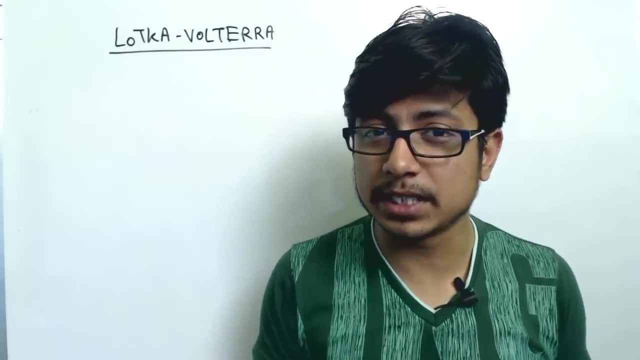 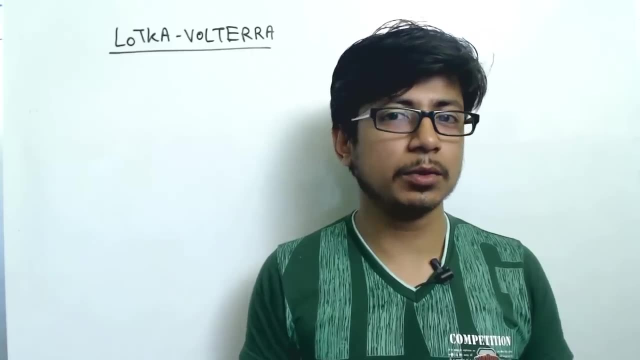 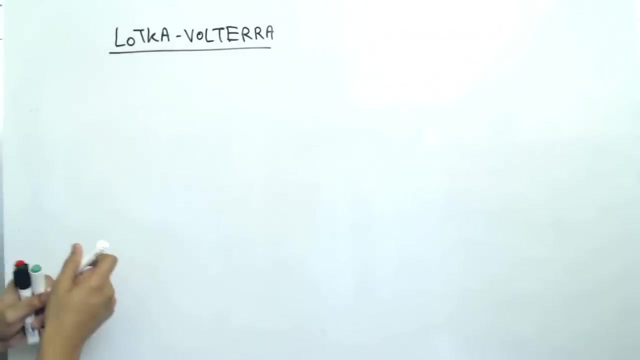 question is: there's a difference between the term habitat and the term ecological niche. Habitat is the place where an organism will live. that concludes with the abiotic factors in that habitat. Okay, that place while niche. so let me write them habitat and Niche ecological. 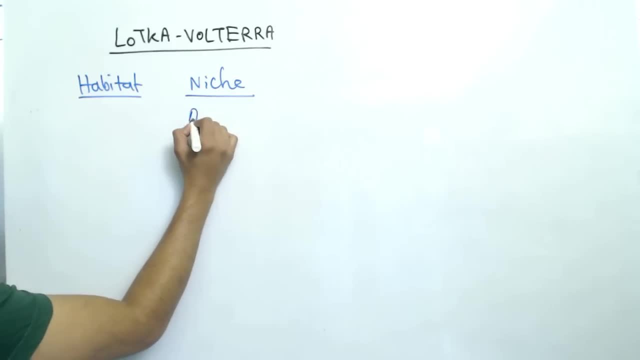 niche This is. it will be the abiotic factor, The food source and habit of the organism all together is a part of the Niche. Niche is much more important to have. This is very important. This is very important If you compare this with the organic, organic animal, organic animal. 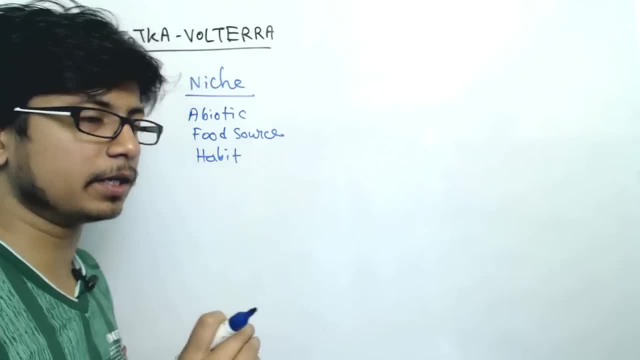 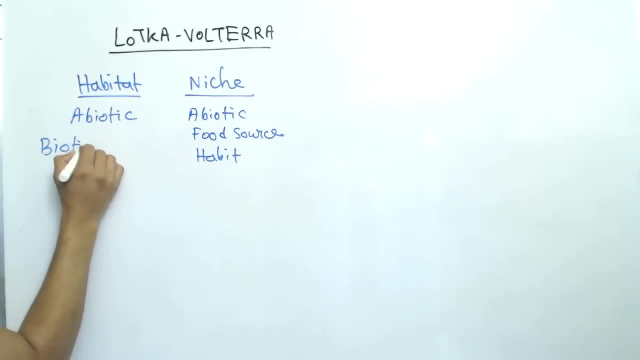 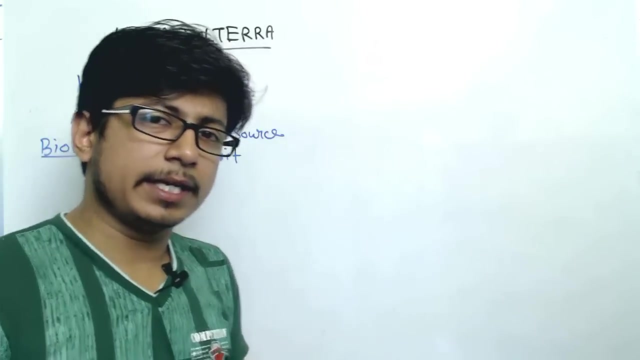 will have the most specific part. It's called the organic. organic organic wild animal. It's much more accurate, much more specific compared to the habitat, which is only consisting of abiotic factors and the biotic elements living there is. if you consider this idea of niche, 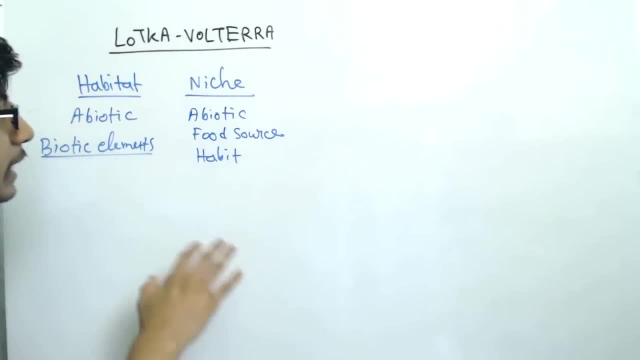 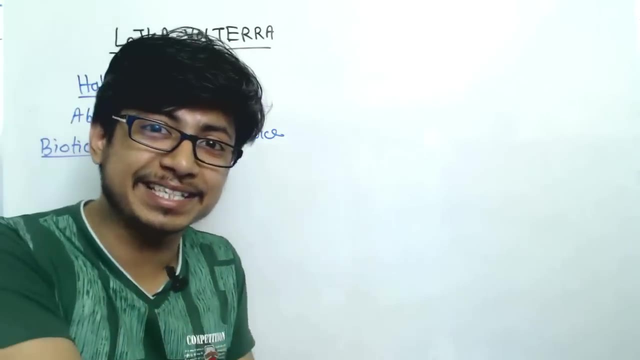 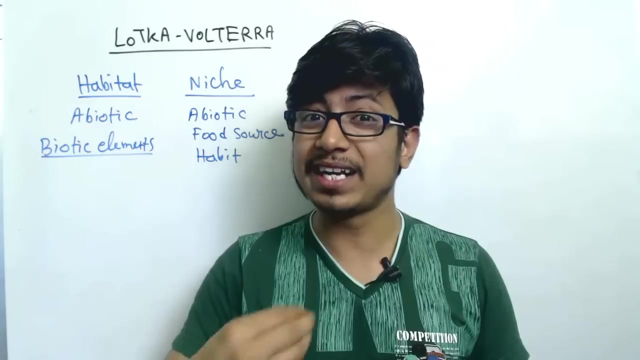 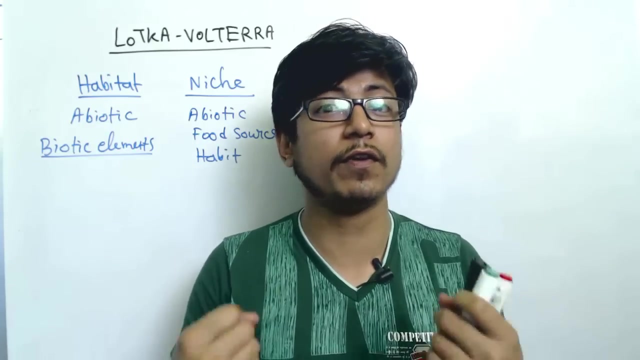 that means an organism's functional role in the ecosystem. that concludes abiotic factor: the food that organism eats right and the other organism who eats this organism right. so for considering niche of mine, that will be all the region that I leave right, what I eat, what eats me, and also my behavior. all those things together will be known as a functional 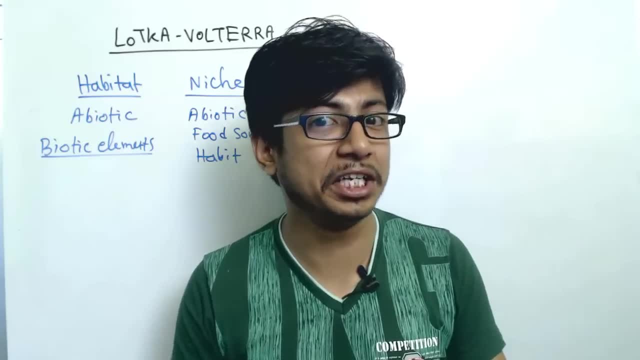 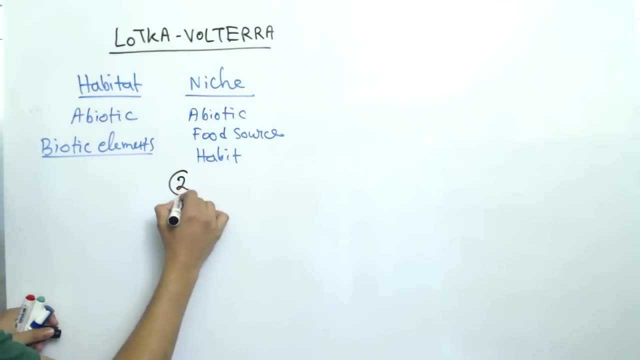 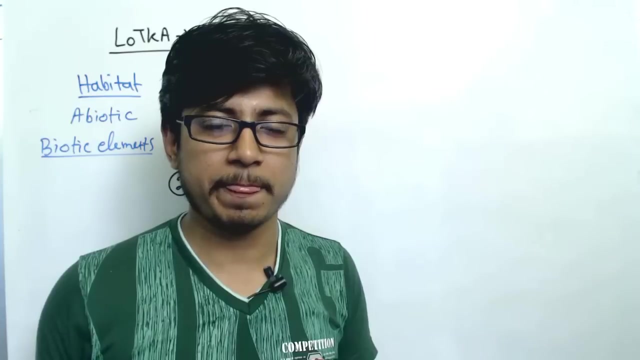 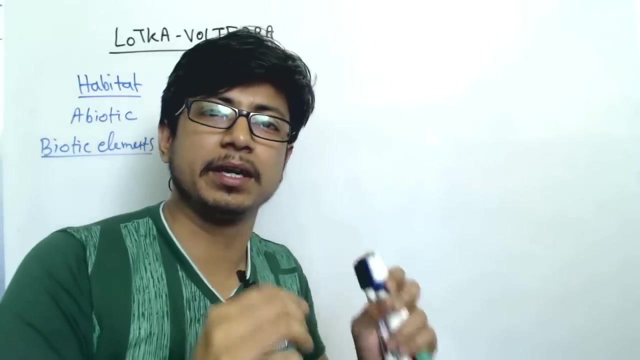 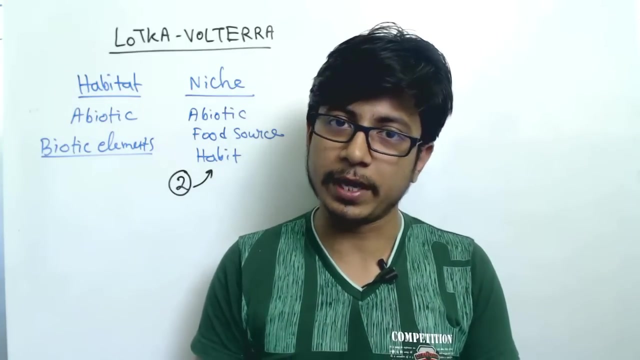 role of mine in that specific region that will be my niche. so if we consider niche, no two species Can coexist in the same niche without ending up in competition. So if two species share same niche then they should ended up in competition. That's the idea known as competitive exclusion principle hypothesis. 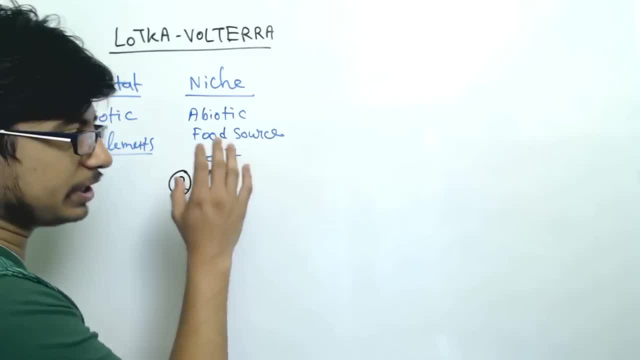 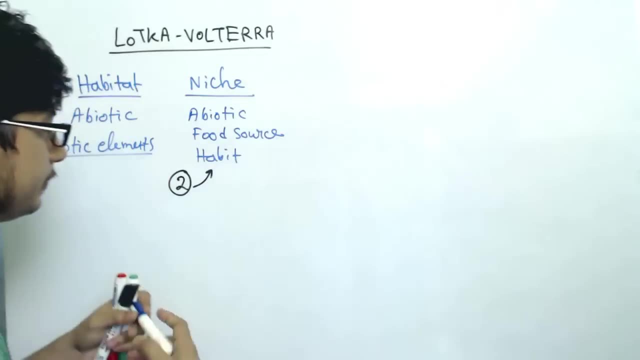 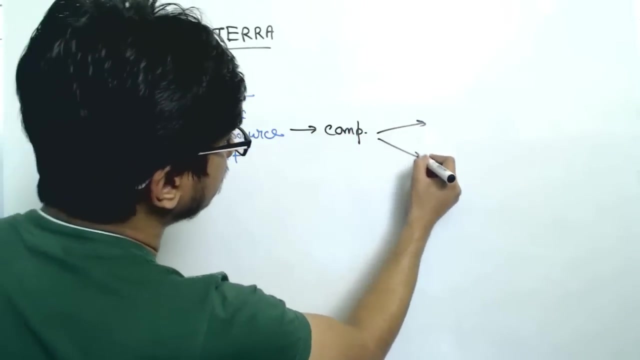 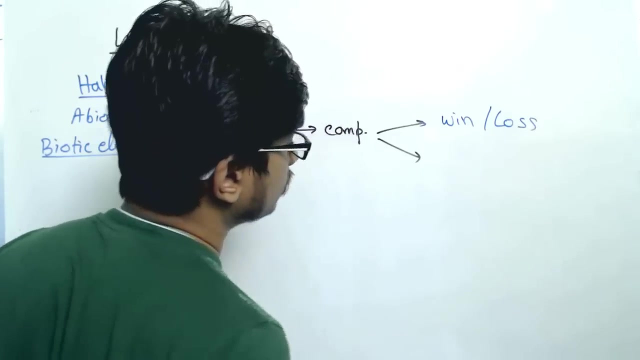 This competitive exclusion principle said that if the niche is same between two species, they will end up in competition. So the result for the competition will be either so the result, so competition will rise. the result of the competition will be one thing we lost. on the other hand, it can be. 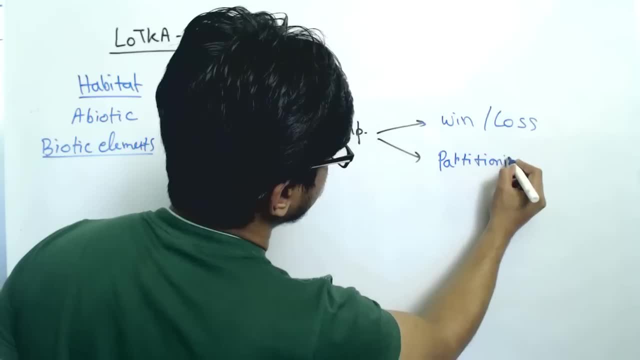 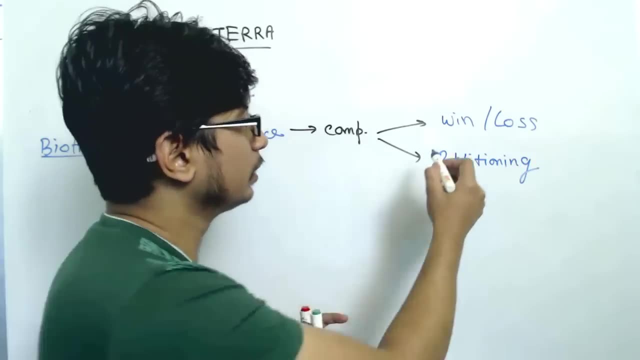 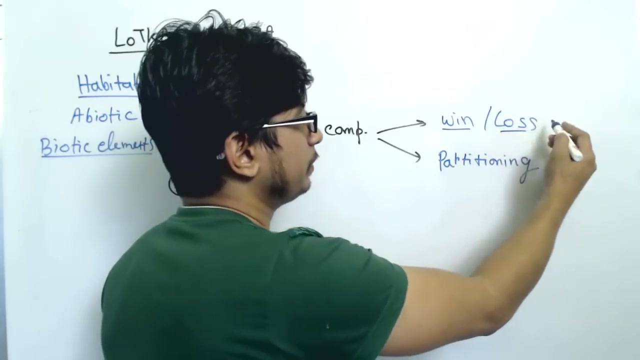 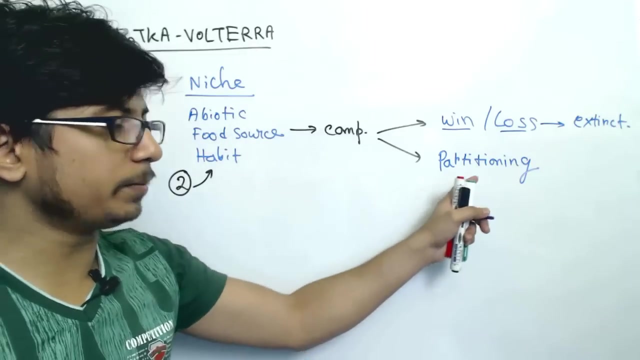 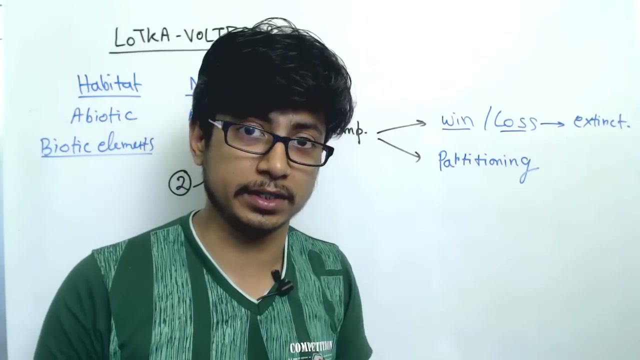 partition, Partition, Partition, Partition, Partition. So between these two species, if the competition arises, one species will win, one will lose. So the species win will live there, the species loses will be locally extinct. On the other hand, partitioning is a way of both the species living belonging to the same niche together in the same habitat. But limiting their resources, That one species- let's say species A, let's say both of them- are bird species living in the same region of the plant, same type of plants and eating same food. So they decide to live in two separate regions of the plant and eating different types of food. 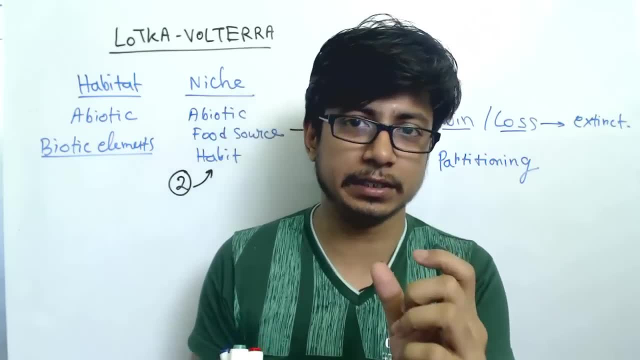 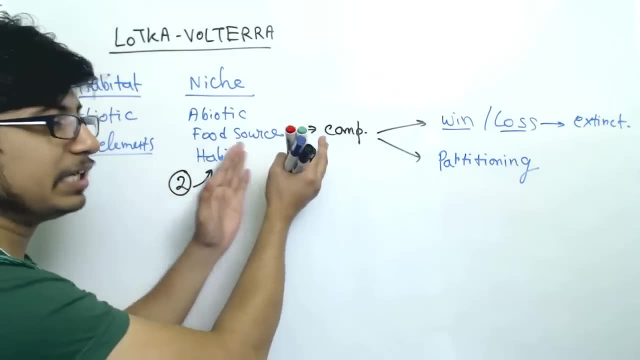 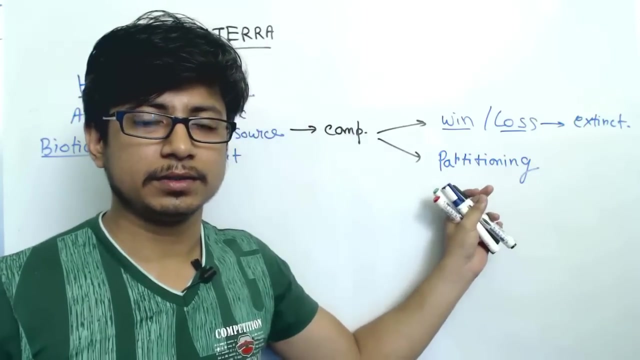 One of the bird is eating only the fruit, another one is eating the seed. By this separation of their food habits they can separate from their niche, So they can form two separate, realized niches that can prevent their competition. That is the term. 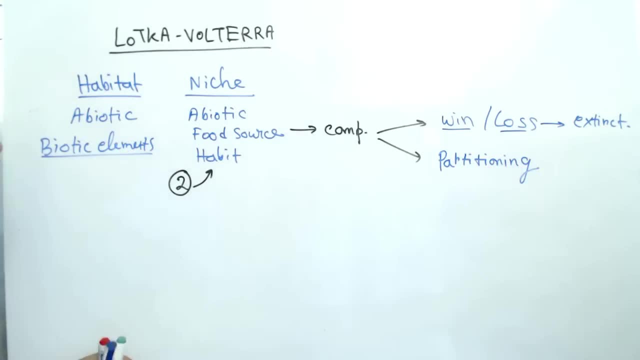 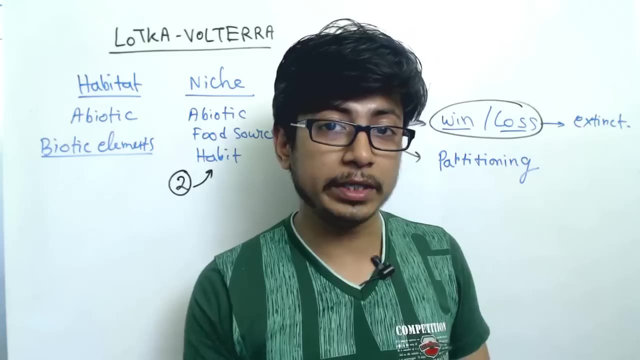 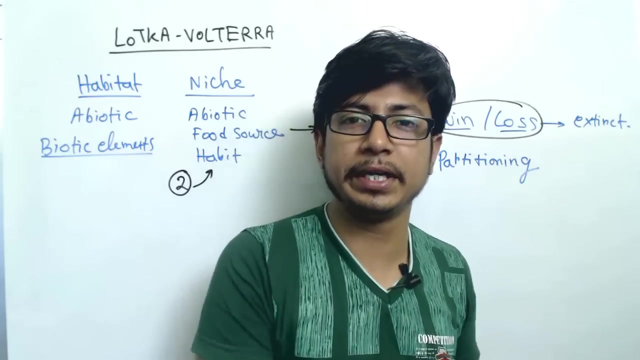 So once you know this idea, we are much interested here to talk about the first situation, when two species are competing against each other. So one will win, one will lose. Whenever two species are competing against each other, then how can we predict the outcome of that competition? 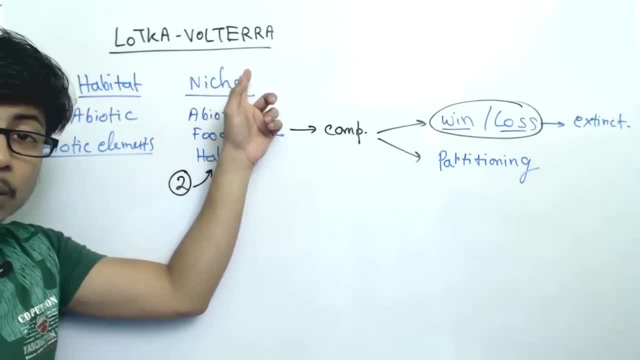 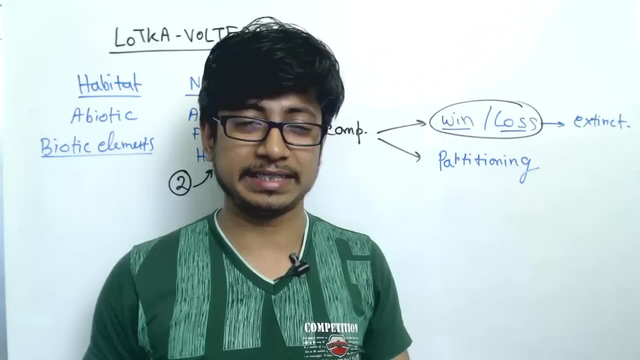 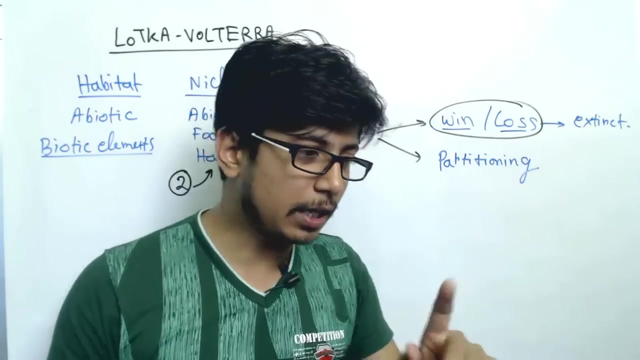 And Lotka-Volterra model. a Lotka-Volterra theory is going to help us predicting the outcome of a competition based on the impact of one species on another. That's what Lotka-Volterra model is all about. So now let's look at here with an example. 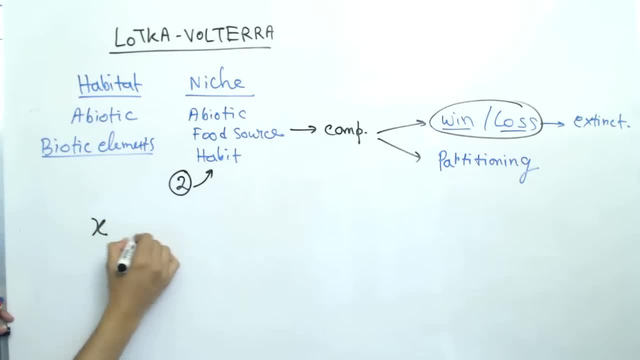 We start with species X and species Y, So both the species are living in the same region. They are ending up in competition. Maybe that they share niche, same niche. That's why they end up in competition. Then what we will see, X will have some impact on Y. 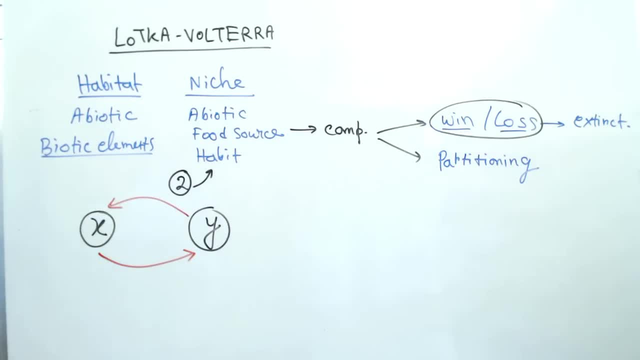 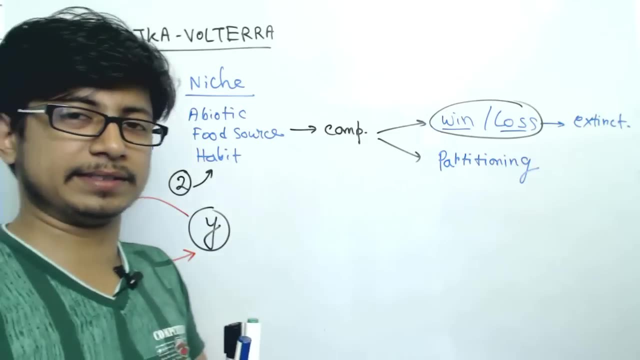 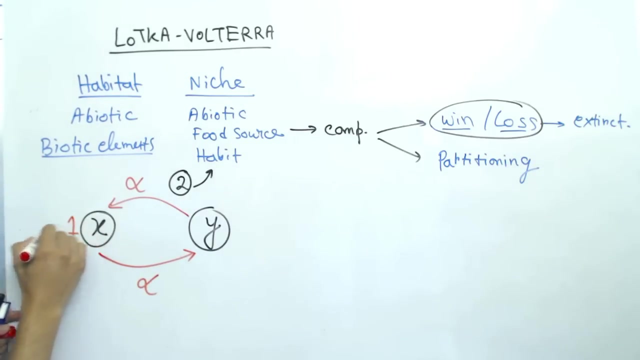 Y also have some impact on X. Now, the impact exerted by X on Y and Y on X is known as a competition coefficient, That is known as alpha Value, known as alpha. We call it species 1. This is, let's say, species 2.. 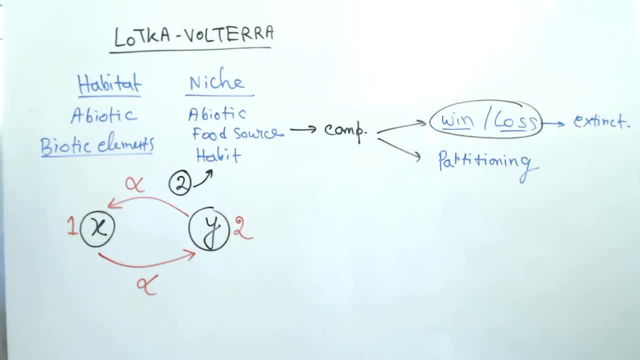 X is species 1 and Y is species 2 in our calculation. So what we can say whenever X is present along with Y, X exerting some competition to Y, And that is known as alpha. But here what we are seeing: 1 exerting the effect on 2.. 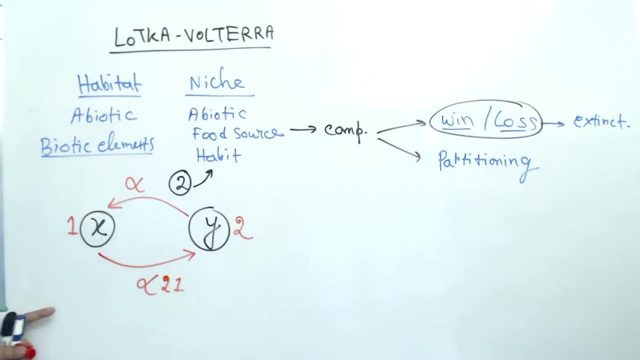 So the value for alpha will be 2, 1. Alpha 21. Alpha 21 means the amount of competition exerted by 2. The amount of competition exerted by species 1 on species 2.. While the other one, the amount of competition exerted by species 2 on species 1, will be known as alpha 12.. 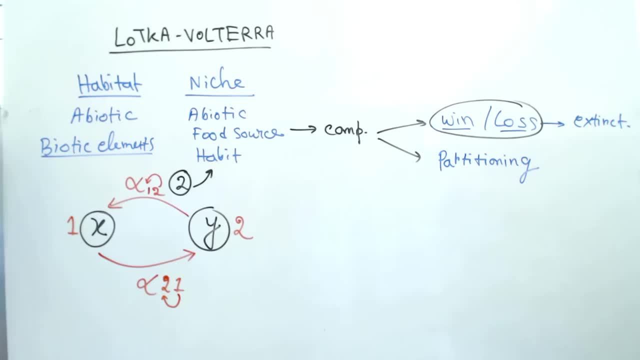 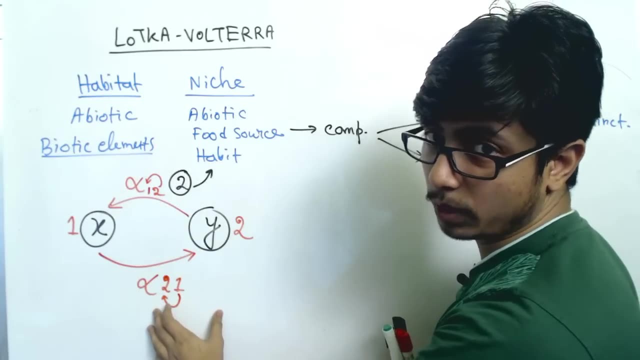 That means competition of 2 on 1.. So that's how we get 2 values. One is known as alpha 12.. Another one is known as alpha 21.. Alpha 12 means the competition of species: 2 on 1.. 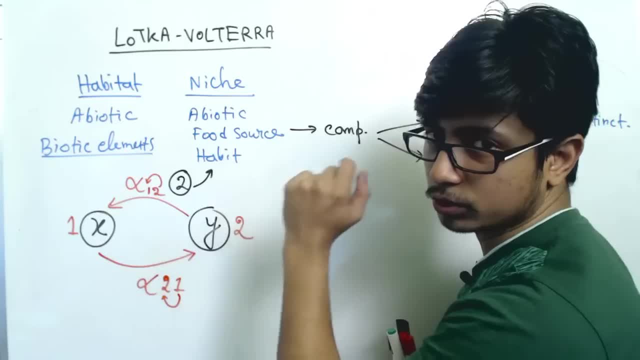 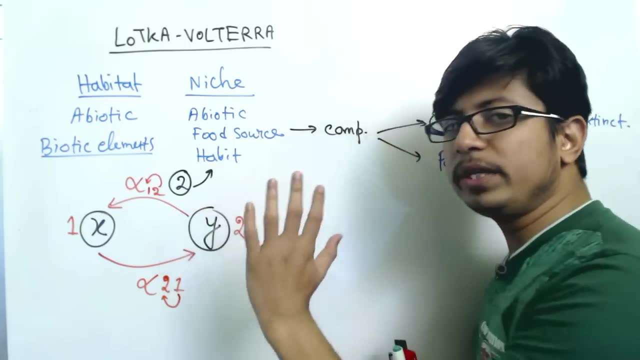 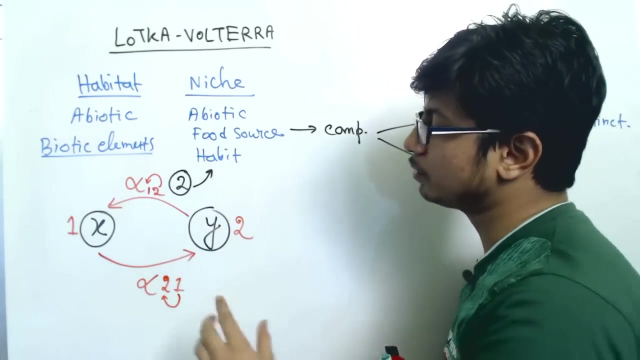 Alpha 21,. competition exerted by species 1 on 2.. So now, once you know this fact, try to analyze one simple thing: If we are trying to know the population growth of species 2. Then we also need to count the species: the population of the species 1 or species X. 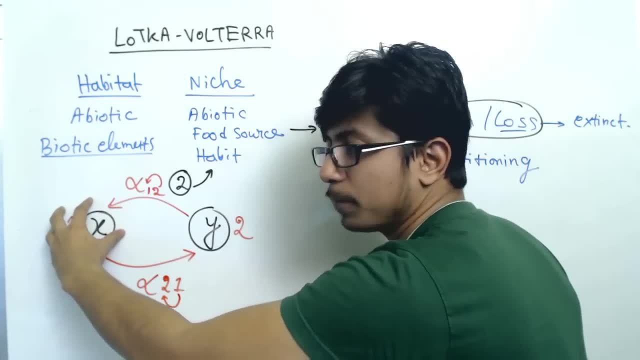 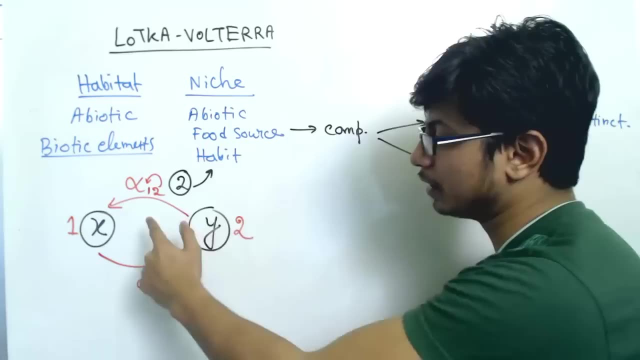 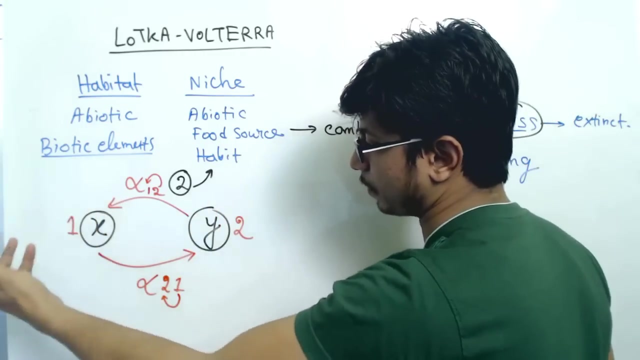 Why? Because if species 1, the size of the population of species 1, if it's more, Then the growth of species 2 will be less due to the competition Right. Similarly, if we are counting the species and the population growth of species 1.. 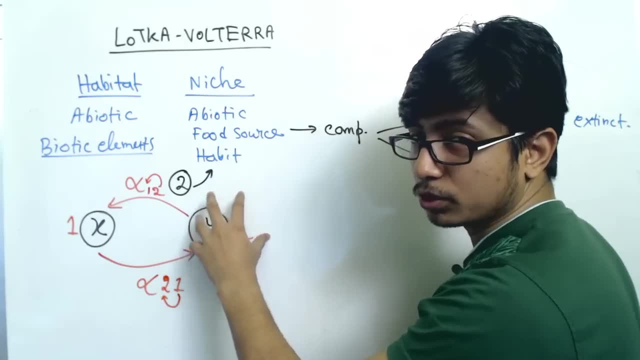 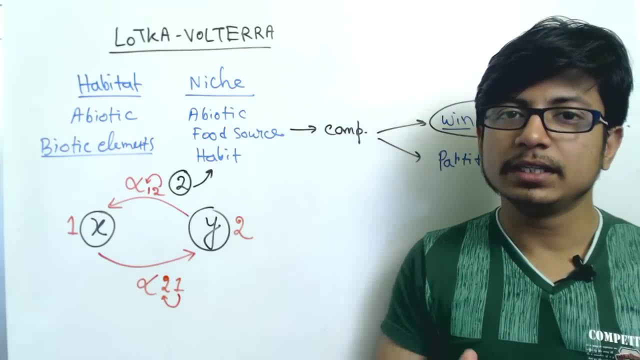 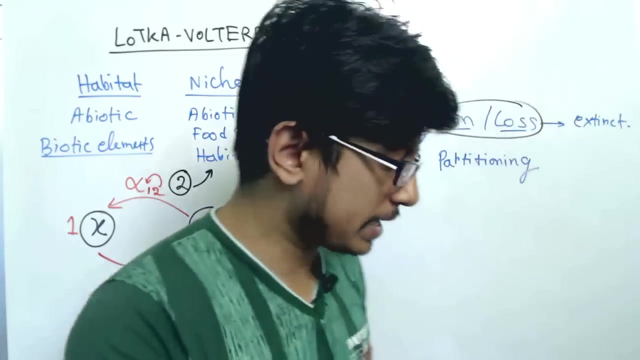 The population size of species 2 also matters. So now we know, according to the formula we can calculate the growth of a population Or intrinsic, we can calculate the growth rate of a population Right Now. if we imagine this growth rate of a population, 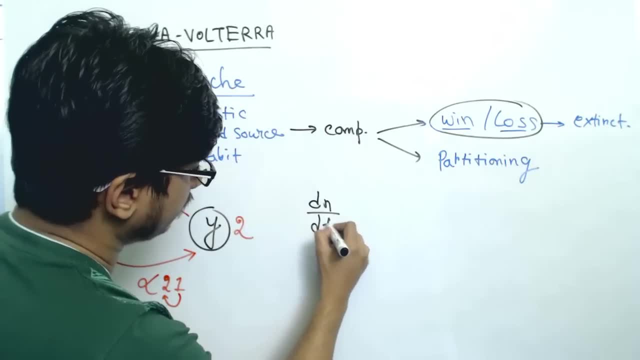 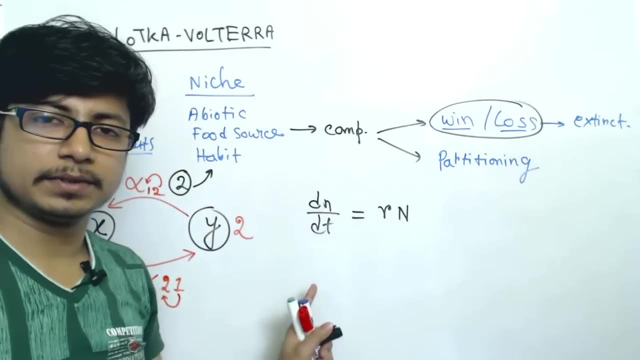 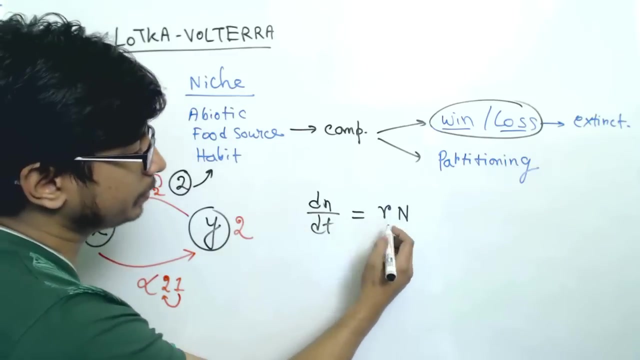 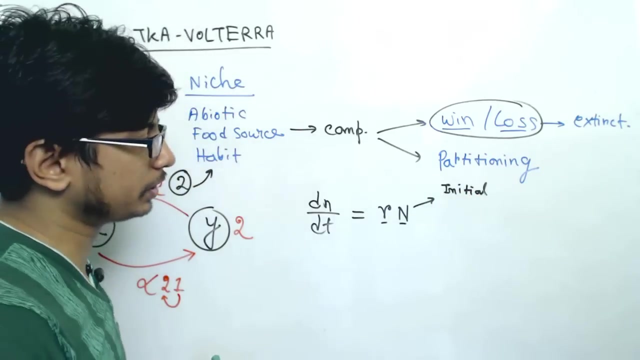 Get to know. DN by DT equals to RN. This is the formula for calculating the growth of a population Right, The total number increasing over time, And that will be RN. N is the initial, initial number of individual of the population Right. 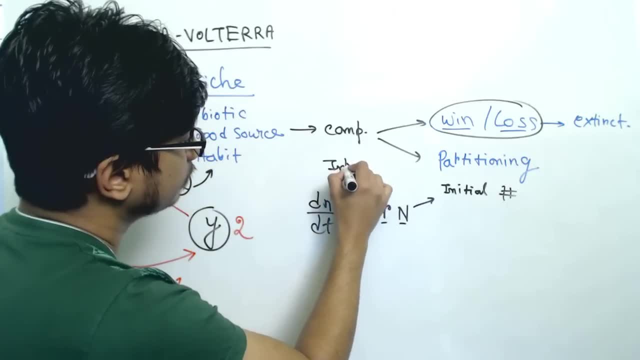 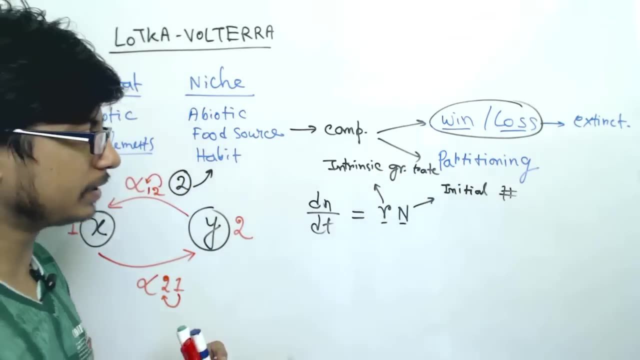 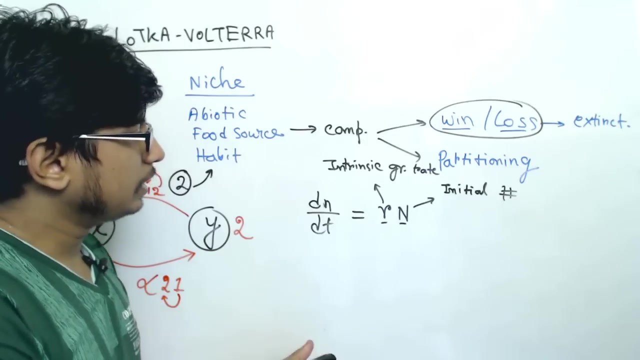 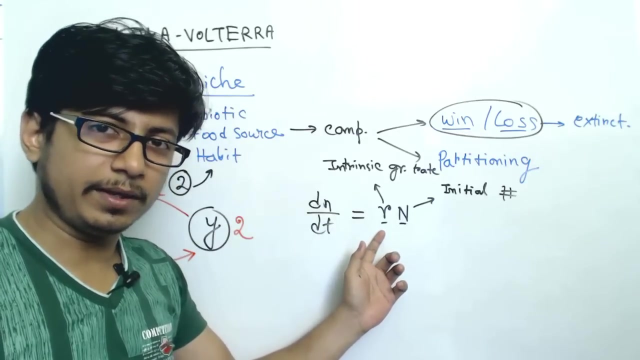 And R is the intrinsic growth rate. Okay, This is the difference. DN by DT equals RN. Now, intrinsic growth rate means it is dependent on birth rate and death rate. So more birth rate, less death rate, R value will increase. Okay. 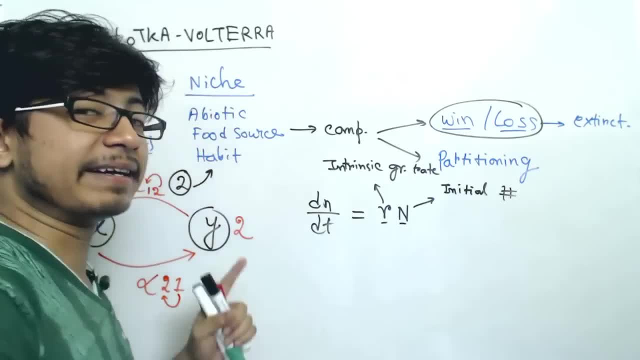 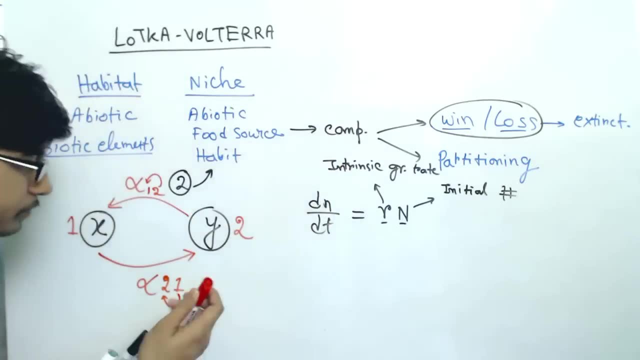 So now, this is the formula for calculating rapid growth. Right, Calculating rapid growth or exponential growth. That's what we know. Okay, This is the general formula Till this point. Let me separate it here. This is the general formula of calculating. 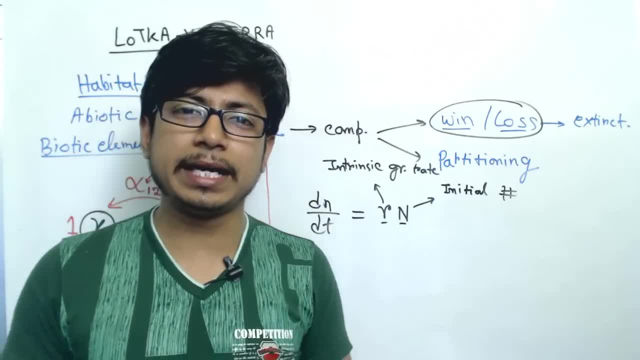 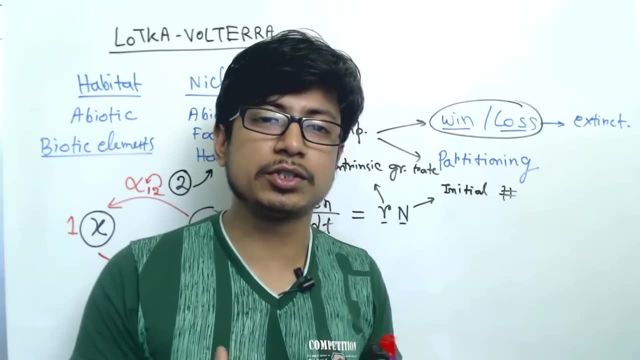 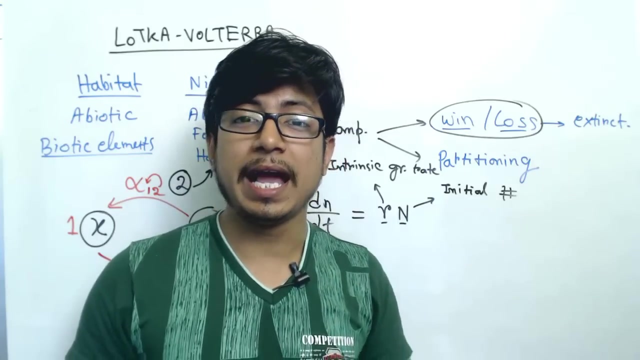 Now, if we do that actually in reality, we know that there is a factor known as carrying capacity. That means an environment's ultimate resource that can support the length of a population. Right Carrying capacity is the total number of individual a specific ecosystem can support for its growth. 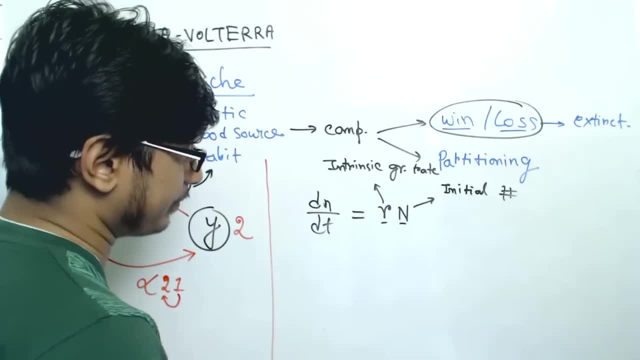 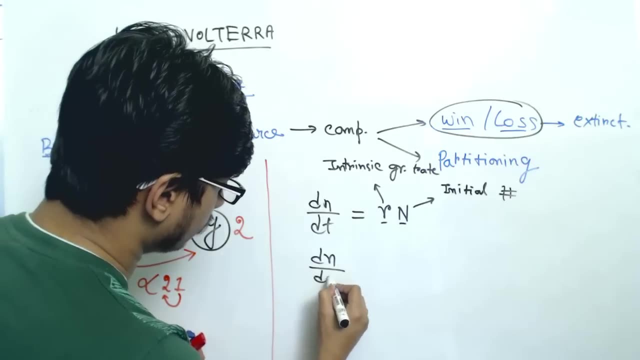 So that is known as key. The value is known as key. So once we take account for the key, we get much accurate. We get much accurate growth rate. So in that case the value will be DN by DT equals to RN. 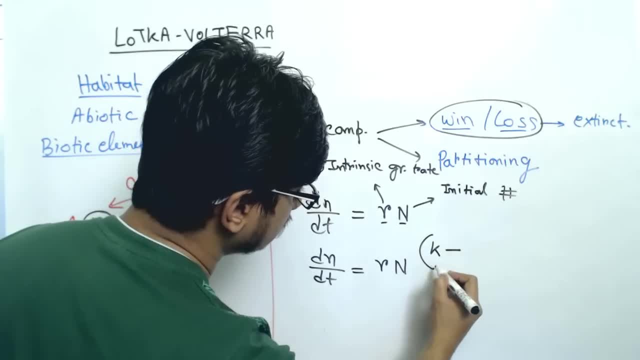 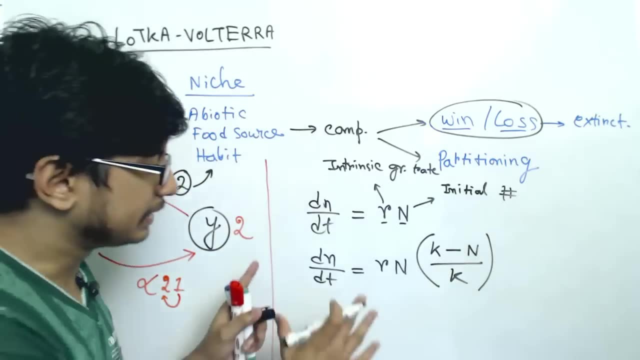 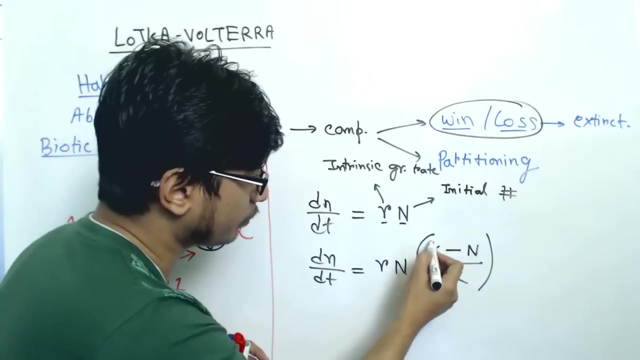 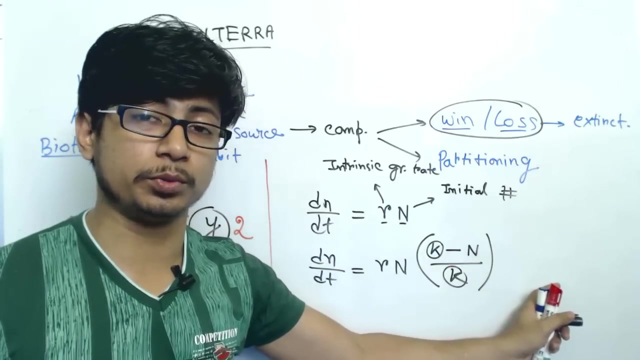 Then what we get? K minus N, Right? This is going to give you more accurate data based on real situations of the wild, because here we take account for the carrying capacity as well. This is going to give us a graph. This is known as logistic growth, which is actually how populations grow, because in the 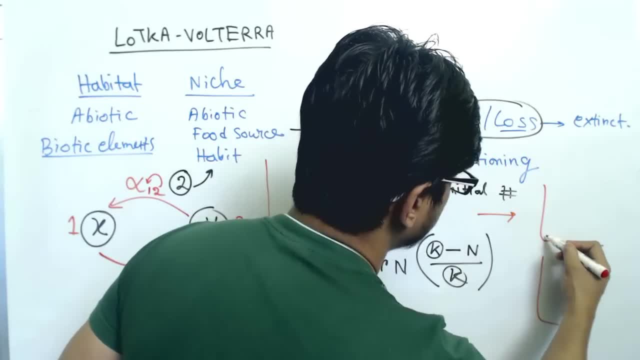 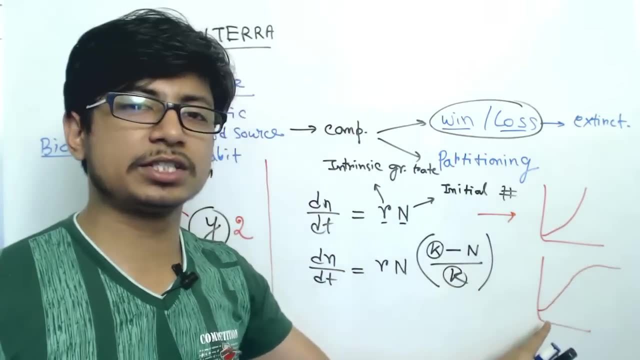 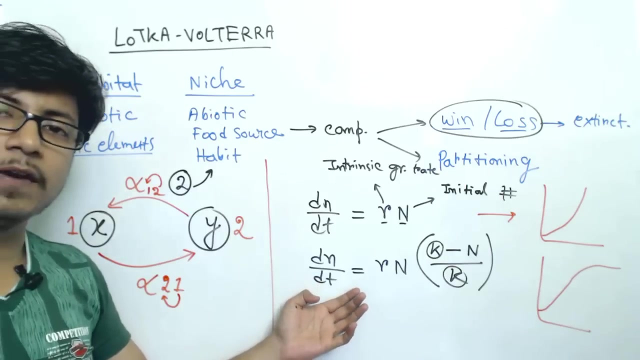 earlier one. this is going to give us a exponential growth. See the growth like this. While this one will give you a growth pattern like this, Logistic growth gives you S-shaped curve and that's kind of reality in nature, But still till this point it's fine to calculate the population growth of one species. 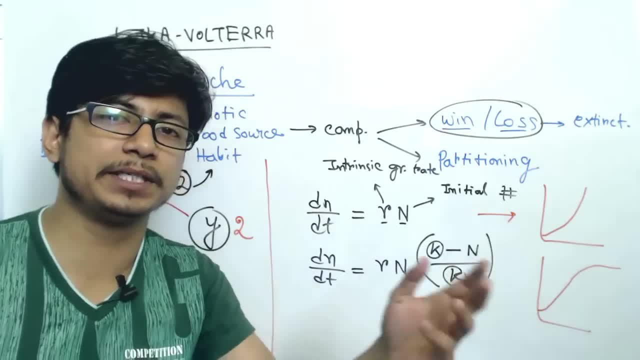 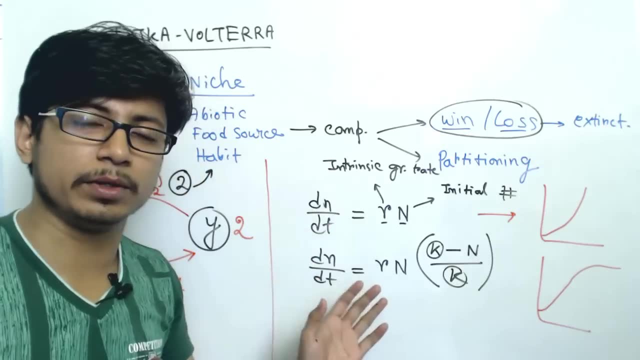 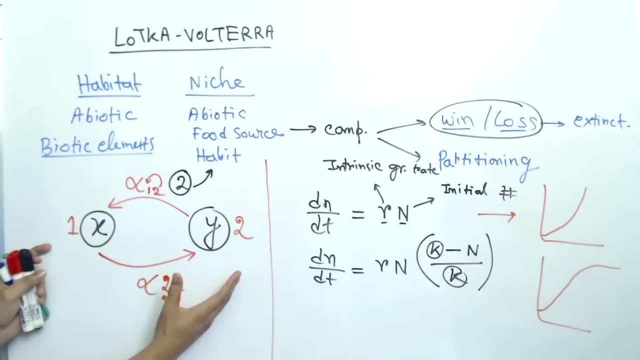 But if that species is in competition with another species in that environment, then how we can calculate the growth of that species? Then this two formula will not be enough to calculate. In that case we need to use the idea of Lotka Volterra model. 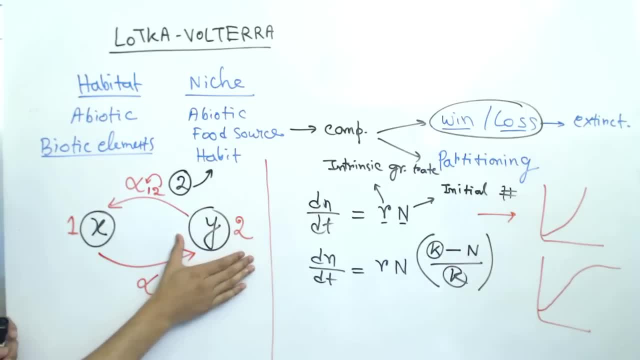 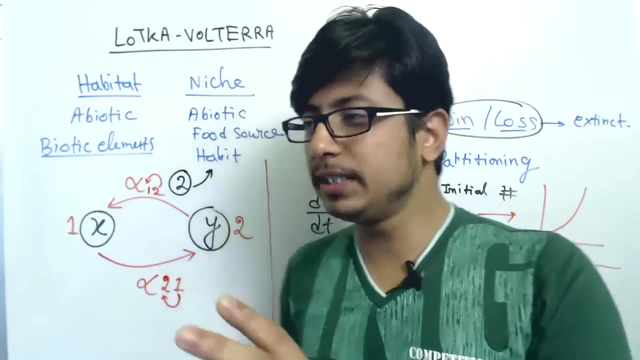 That is, if we are calculating for one species which is in competition with other, we need to also take account the population size of the other species and many other factors. We call it predator prey model. Why we call it predator prey model? because in this competition we know one of the species. 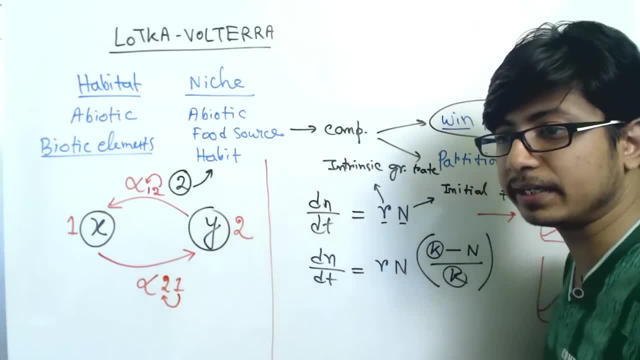 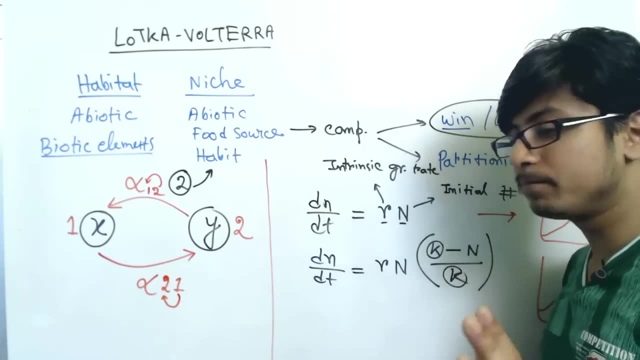 will win. One species is more impactful, That will be known as a predator, while the other one will lose, less impactful, known as the prey. That is the idea. So once we check the total number of predator and prey in the population, then we can tell. 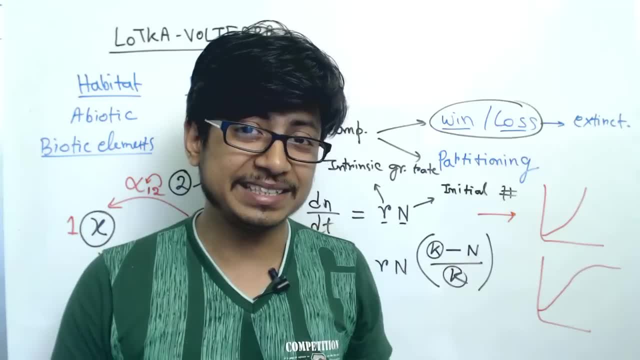 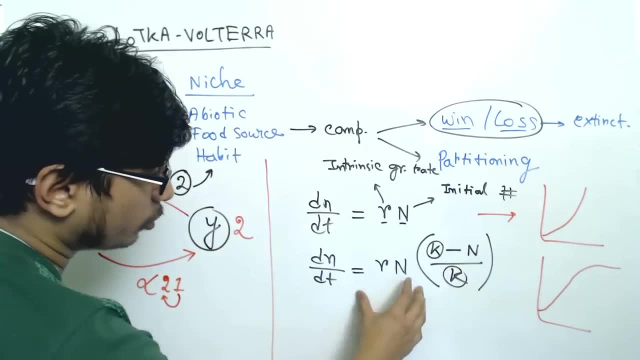 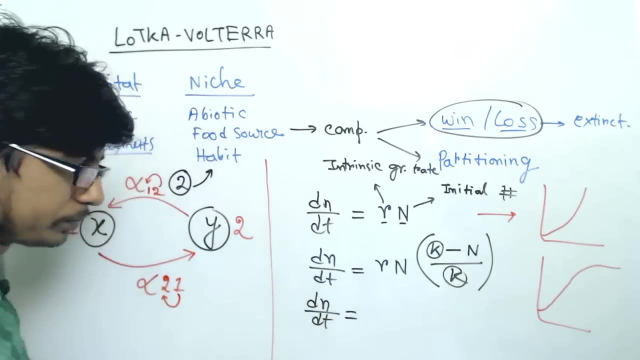 what is going to be the outcome and what will be the growth rate of either predator or prey in the environment. So for that to calculate, we need to tweak this equation a little bit, and the change that we need to bring is now: DN by DT equals to: 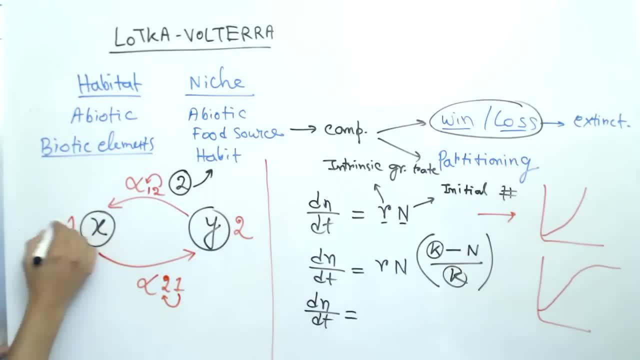 Let's say, here we are calculating the growth for species one in presence of species two. So if you're calculating the growth of species one, let's say the total number of individual present at the beginning of species one is in one and species two is in two. 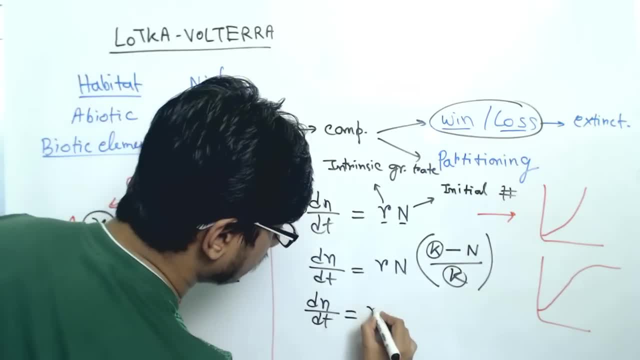 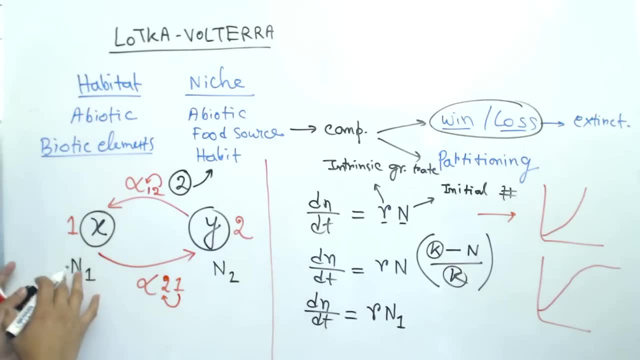 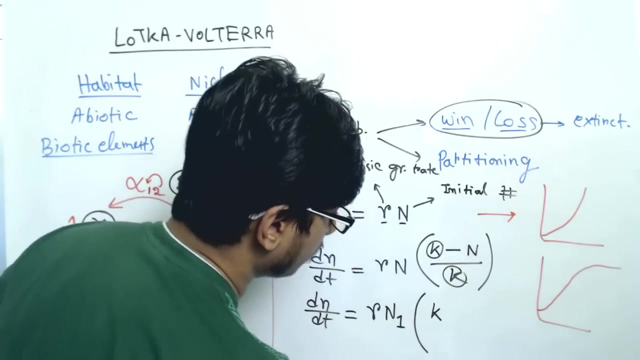 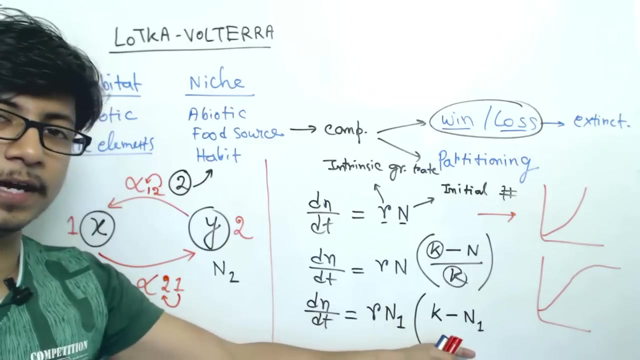 So if you go with in one, so what we get- intrinsic growth rate are individual rate in one, because we're calculating the growth rate of species one, So it will be our in one. in the bracket It begins with K minus in one. Okay, that is still this value. 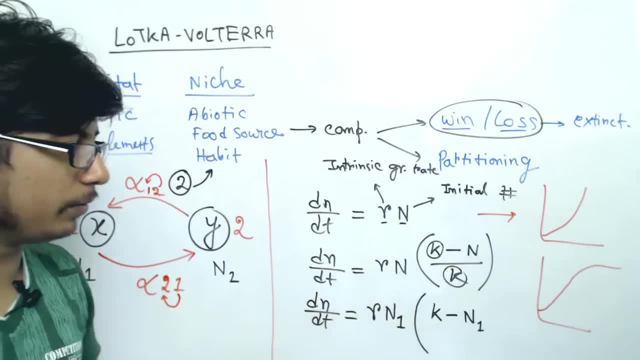 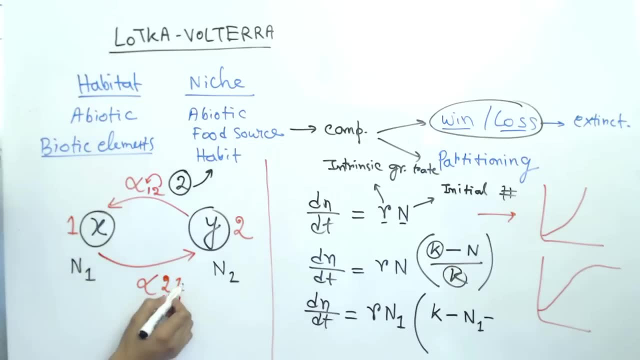 We have the similarity with the logistic growth, but now we will see minus. we have another value here, Another parameter, that is, the impact of one species And in this case, what we will see. we are trying to calculate the growth rate of species one. 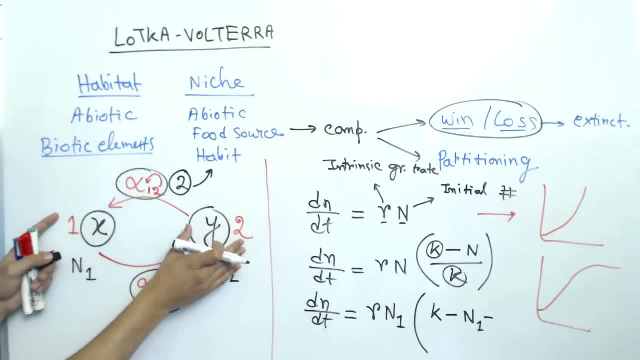 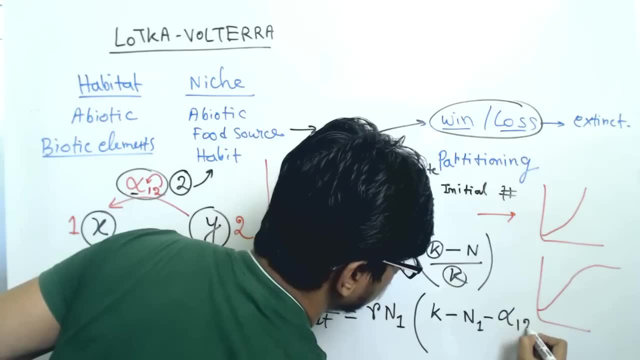 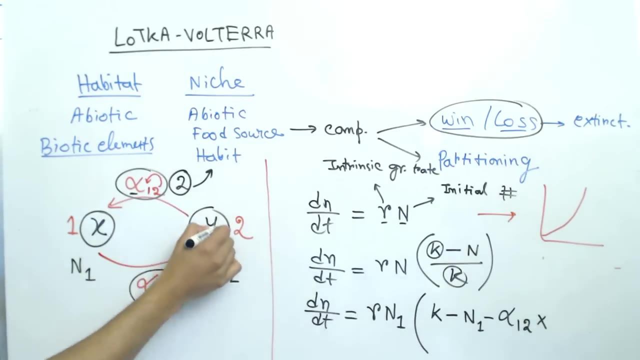 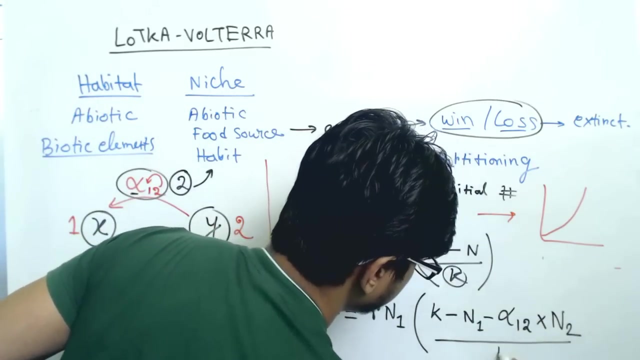 So the impact that we calculate will be the impact of species two on one will get the value of alpha 12.. So alpha 12 into the total number of individual present in species two, that is, in two divided by K. So what we get here is this value. 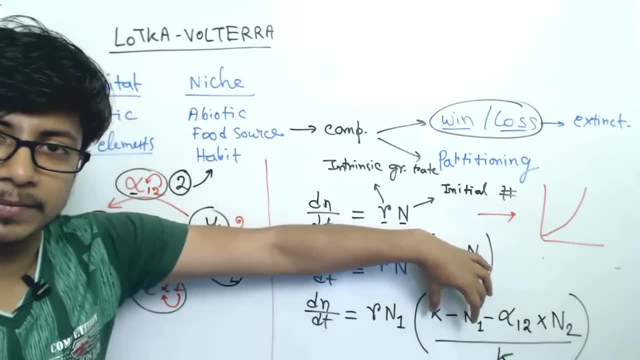 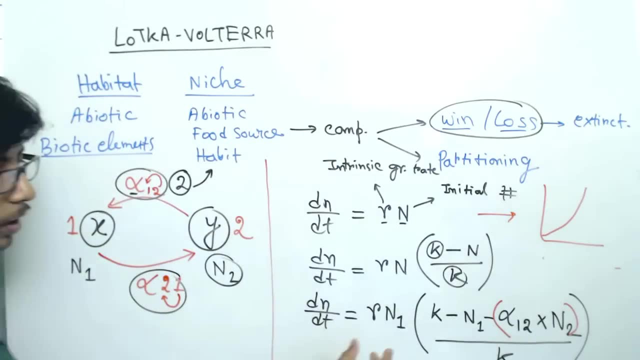 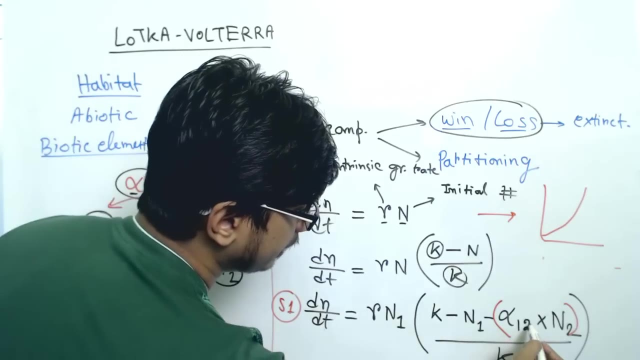 Right. So remember till this point, the value is same, like the logistic growth. Only these two portions are different. This equation is only different. Why? Because we are calculating the growth of species one, So what. we want to calculate the impact of species two on one. 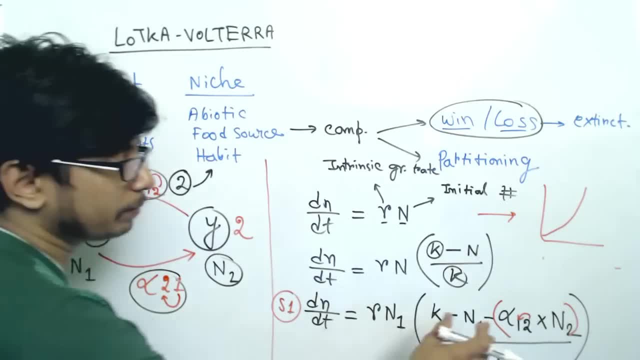 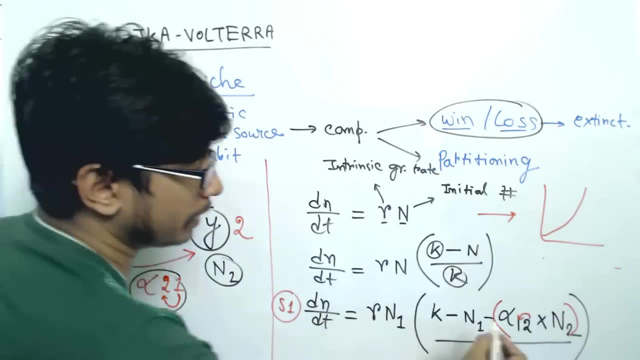 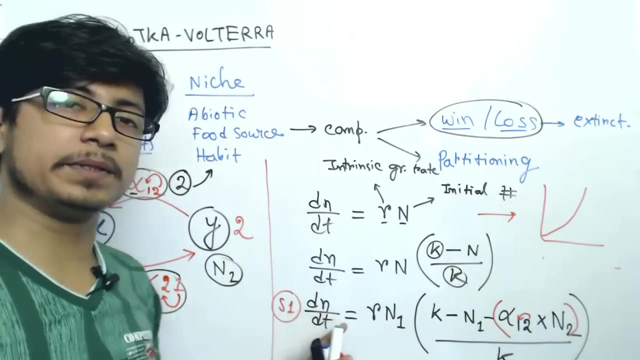 And that impact will be further if the number of species two is more. So we need to also take account for the total number of individuals present in species two, So multiplied with n two. That's how we get the formula to calculate the growth of species one in presence of species. 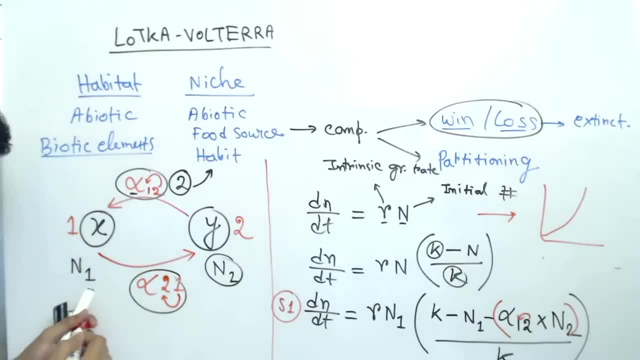 two. Okay, Similarly we can do that for another one, for species two. Now dn by K, dn by dt equals to our n two, Then carrying capacity minus into minus. here we are calculating the growth of species two. So growth of species two means we want to check the impact of species one on two. 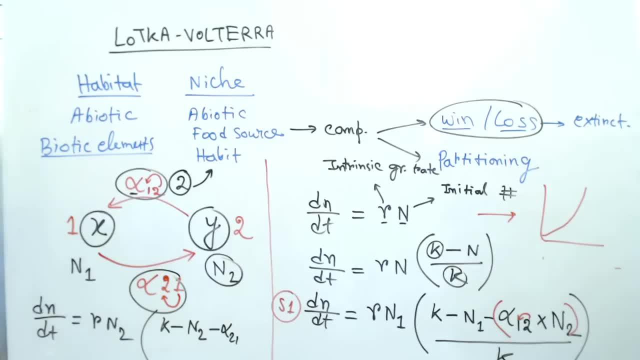 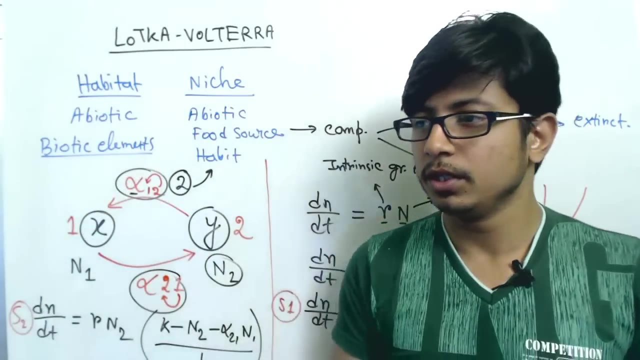 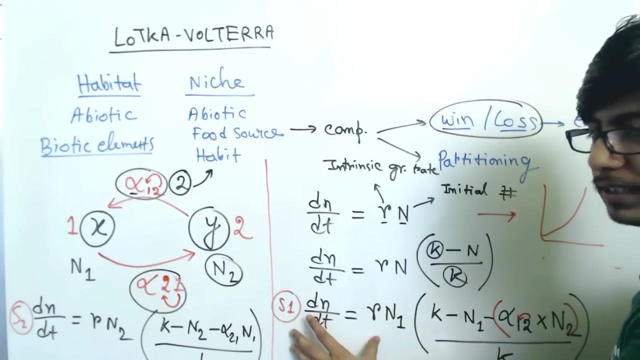 So that is alpha 21 into the total number of individual of species one divided by K. So this is going to give you the growth of species two. So what we see now, in both this case we are able to calculating either the growth of species one or the growth of species two, correctly involving the idea of Lotka Volterra model. 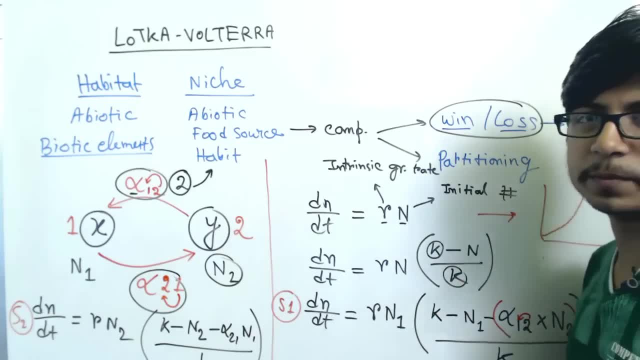 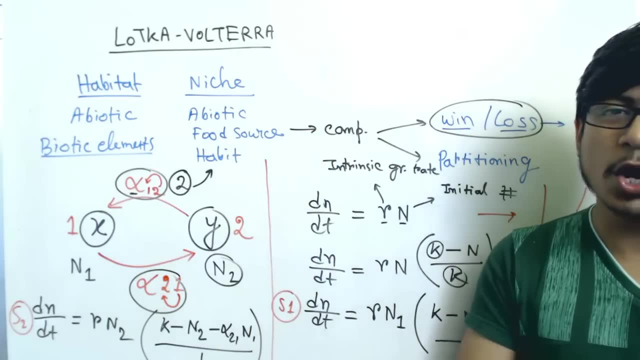 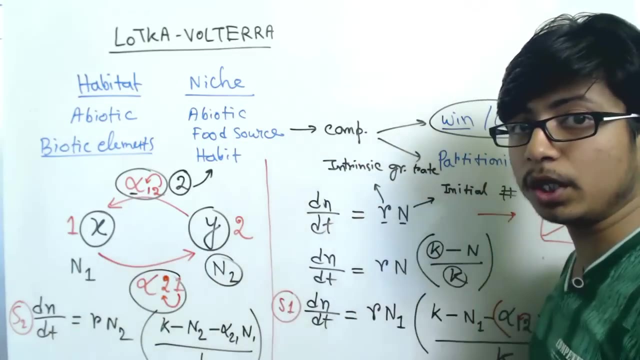 So in reality, always the competition is present. in many cases in the wild, If you look, there is competition, intraspecific competition, all around it. They are present. So in reality, we always need to take account for this Lotka Volterra model to calculate the growth rate of one species in presence of the other. 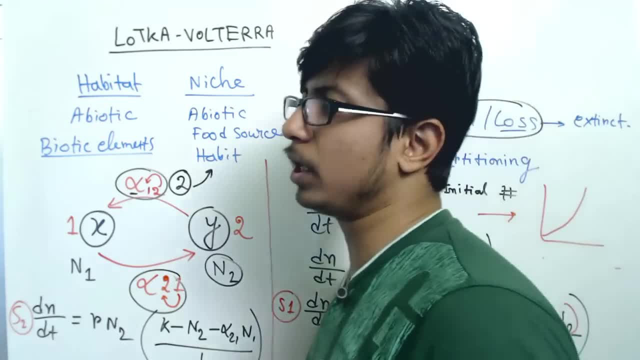 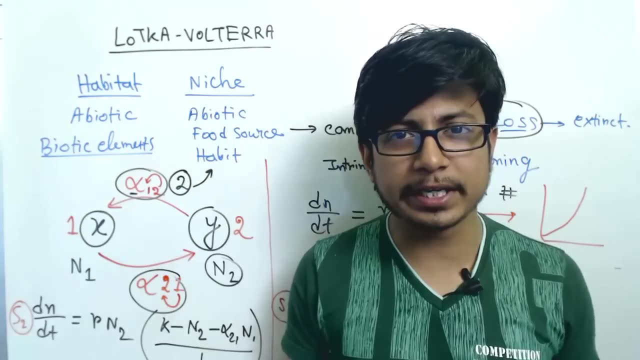 Now this is only one part of Lotka Volterra model. Now the question is- I told you at the beginning, between the competition of two species, Can you predict the outcome of the competition? The answer says yes With Lotka Volterra model. 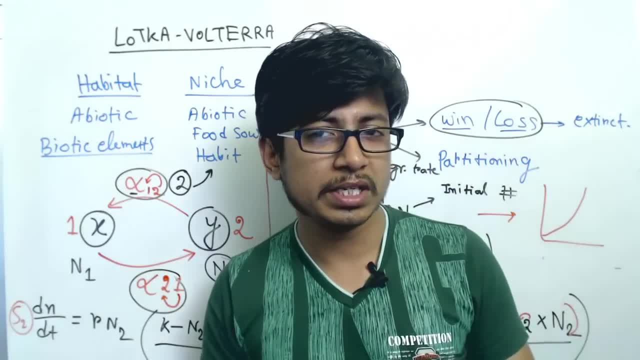 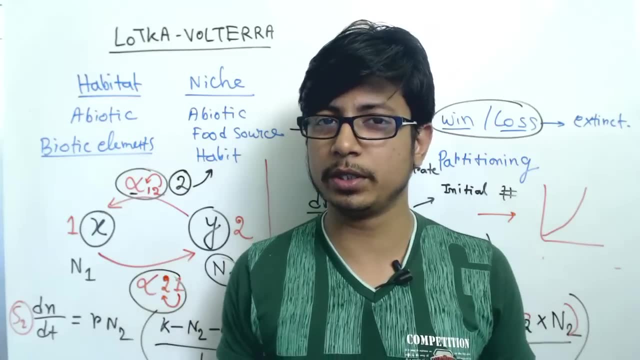 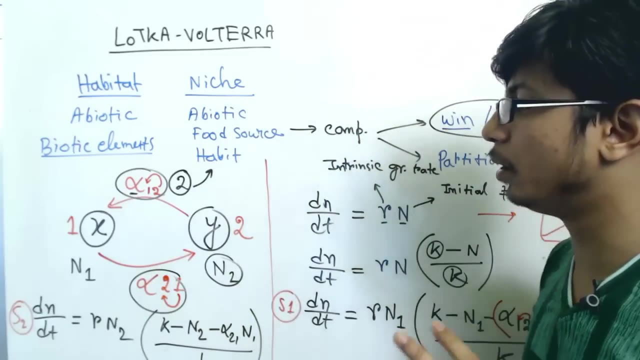 we can predict the outcome of the competition model. we can achieve that to. the question is: how can you achieve that idea, whether between species one and two, who is going to win and who is going to lose? to get the idea about that, we need to construct a graph using the value of the n one and n two and also calculating. 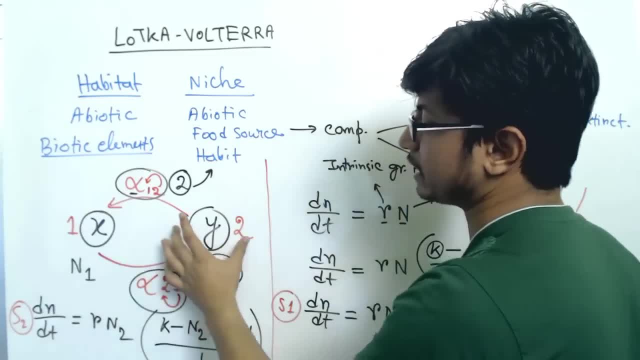 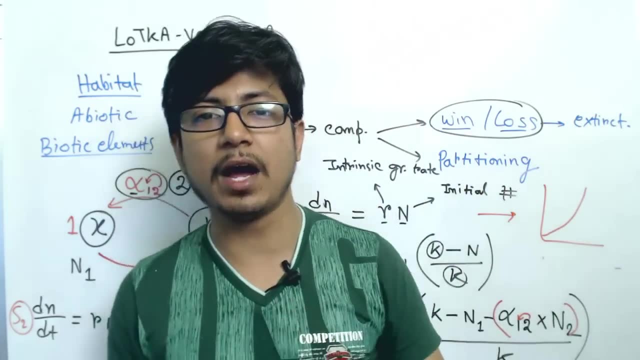 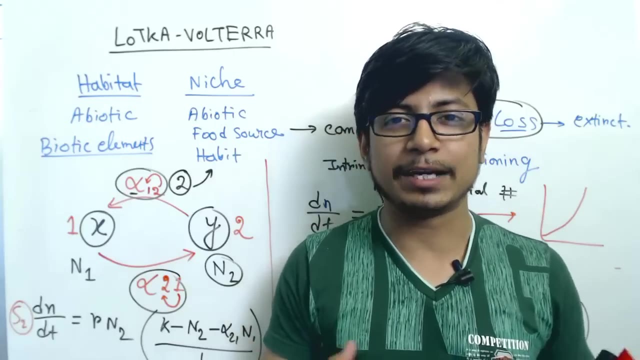 the carrying capacity of both species one and species to- in presence of the opponent species. that's going to give us a graph and with the help of that graph, looking at the pattern of the graph, we can calculate between species one and two, who is going to win and 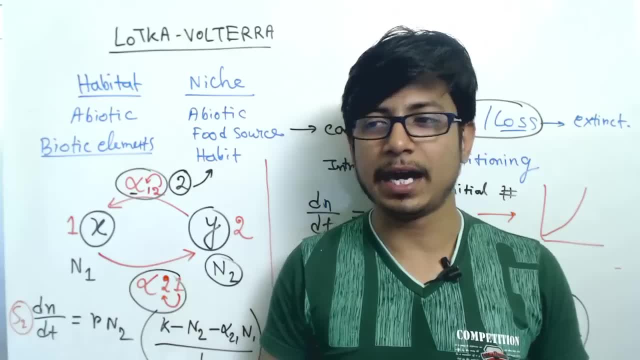 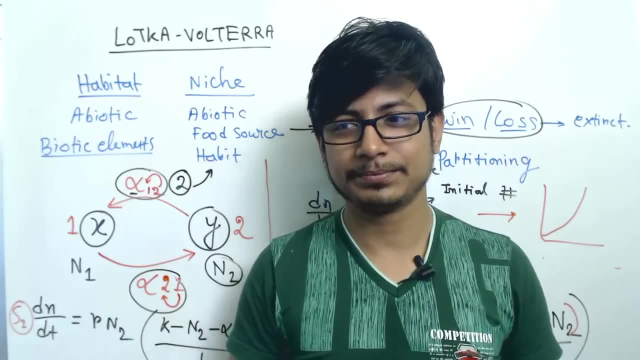 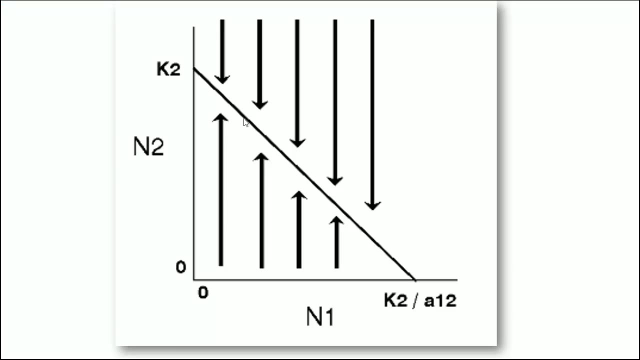 who is going to lose. Okay, so let's look at it. I have those graphs in my computer, so I'll go back to my computer to show you how do you calculate that outcome. Okay, so now, as we know about the Lotka Volterra model, here we will see how to predict the outcome of a competition. 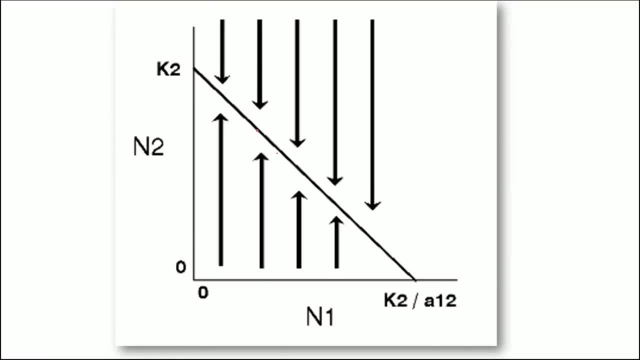 involving the idea of Lotka Volterra, to understand that you need to know this graph, As I mentioned you earlier that in this graph we have in one index axis and into the y axis. in one is the number of individual to start with for species one and into is the initial number. 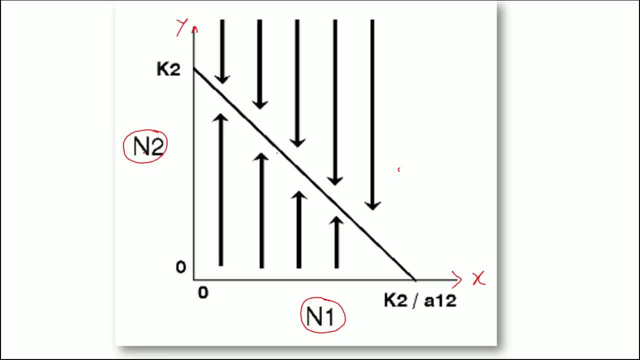 of population size: initial number of individuals in the population for species two. Now, I also told you earlier regarding the value for K, which is carrying capacity, and we know carrying capacity can be calculated based on the total number of individuals supported by the resources provided by the environment. so carrying capacity should be the maximum. 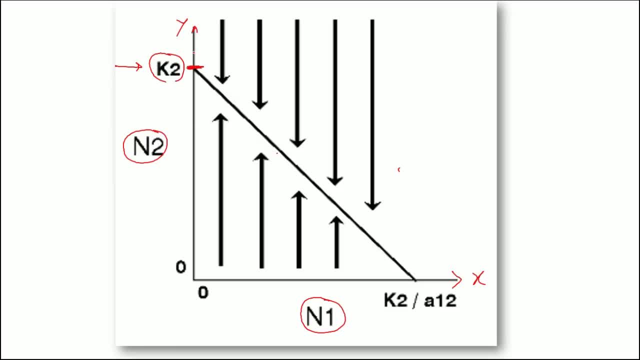 number of individuals supported in this case, which is also depicted in y axis. Now the thing is, while we are calculating the carrying capacity of K two, that is, the carrying capacity of species Two, we need to take account the presence of species one of the number of individuals. 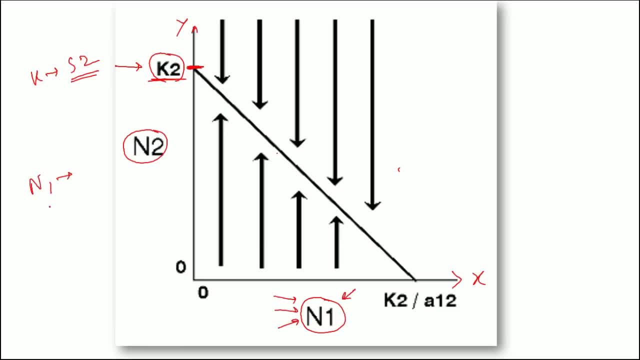 present in species one. This is one thing, and the second thing is the alpha 12, that is the impact of species 211.. In this case, normally we need alpha 21, in which is the impact of species one of species two. So, while we are calculating the carrying capacity, 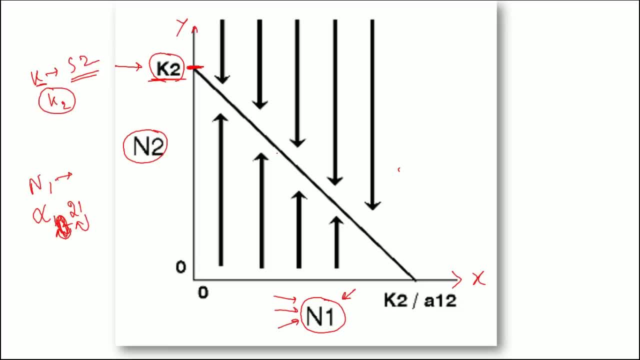 of species two or K two. we want to calculate for the number of individuals supported by the resource. We are going to implement alpha 11 in this case, because a lot of these things are not involved in actually carrying capacity, because alpha 11 is the number of the species. 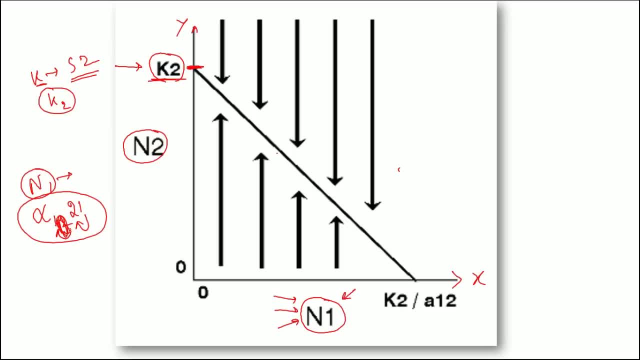 Alpha 11 is the number of individuals of species one and the impact of species one on species to both of those things matter. and also alpha 12,, that is the amount of impact or provided by species to on species one. So now, if alpha 21 is greater than alpha 12,, then what will? 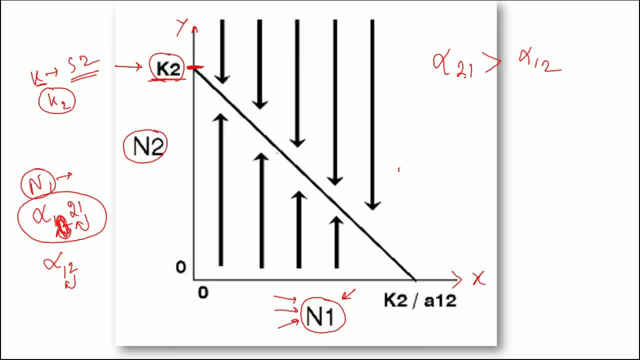 happen. That means the impact of species one and two is far greater. The impact off it is two and one. So in that case the carrying capacity value will be less. if the initial number of individual of species one is high, is that clear? So in one is high and the value for alpha 21. 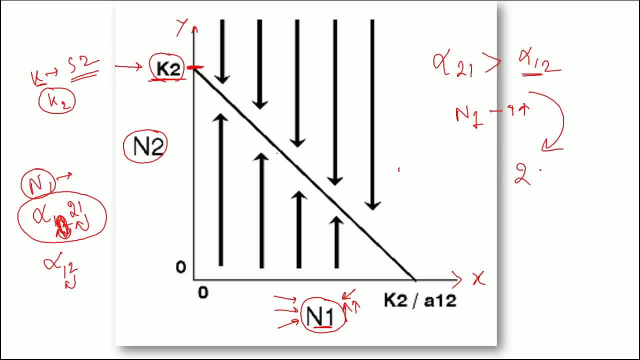 is greater than alpha 12.. That means two will use right, one will win. That is the idea. Okay, Now the similar thing. if value for alpha 12 is greater than alpha 21 and number of individual present, initial number of individuals in species one is less, that means far less impact provided. 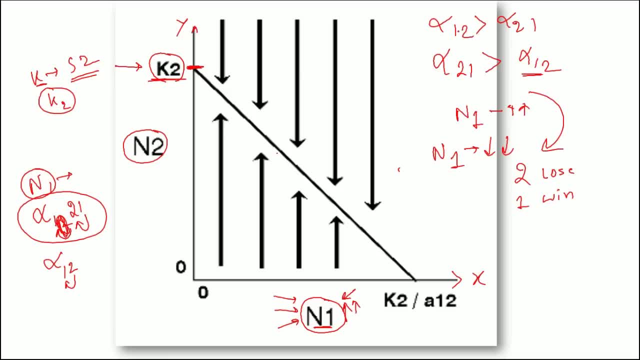 by species, one on species. So normally the impact provided by species 211 is high, So the carrying capacity of the K2 value will reach maximum. in that case K2 will be high and species two will win. This is how we can calculate whether species one will win or species two win will. So now 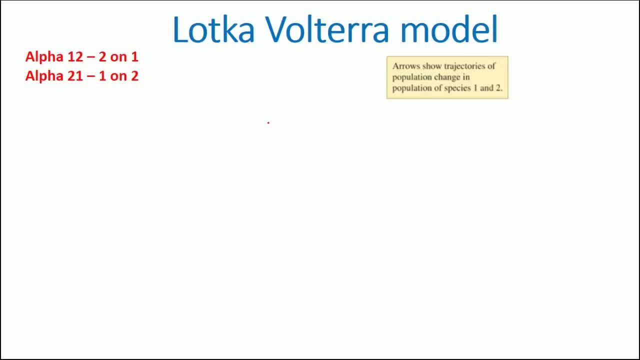 let us look at here in the two, three separate graphs of how we are calculating it. In this first graph, what we are seeing is a calculation of parallel graphs for both species two and species one. The graph with black color is a species two and the growth pattern. 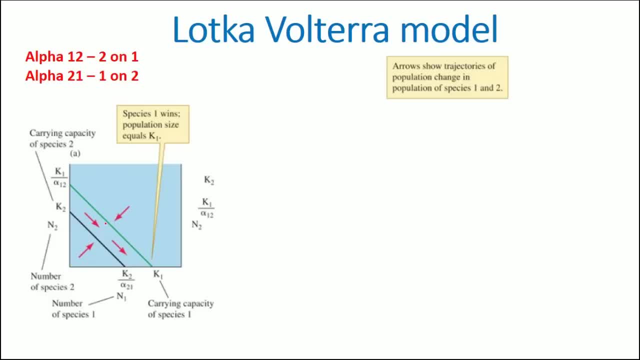 of species two, and the green one is for the growth pattern of species one. What we are seeing here is that the value for alpha and the value for alpha 21 and value for alpha 12, right, So here, So here. 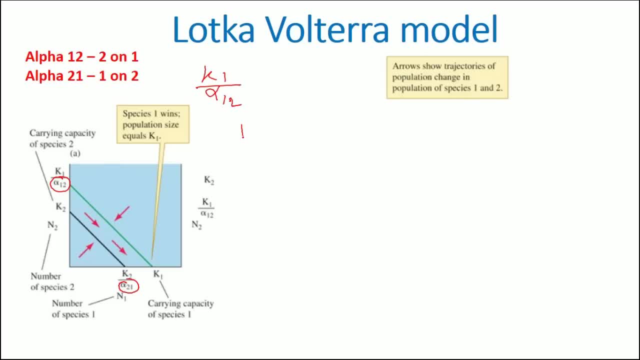 So, as we see the value of K1 by alpha 12, another one is K2 by alpha 21.. Now just imagine if the value for alpha 21 greater than alpha 12, then what will happen? This value will go less and the value K1 by alpha 12 will increase. So what we will see As a result. 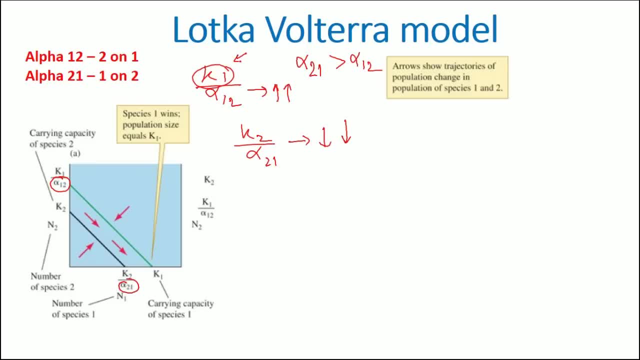 the carrying capacity for one species one will increase Here. This will be the carrying capacity of species one, which is increased due to low alpha 12.. But as alpha 21 is high, the carrying capacity for species two is decreased. So you see, if we now calculate the carrying capacity for alpha for species one is this: 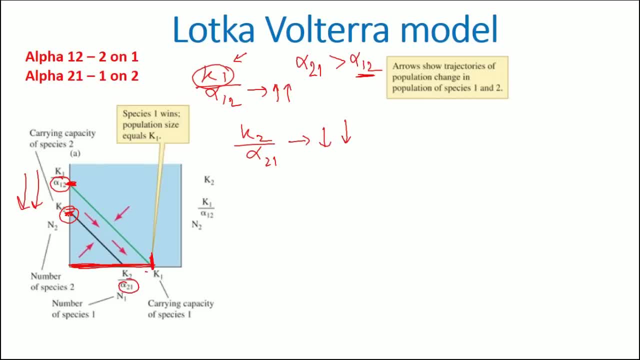 length And the carrying capacity for species two is only this length. So, as we see, carrying capacity of one is further increased of carrying capacity of two. That means we know, with the same resources, more species one can leave and the environment can support more K1. So 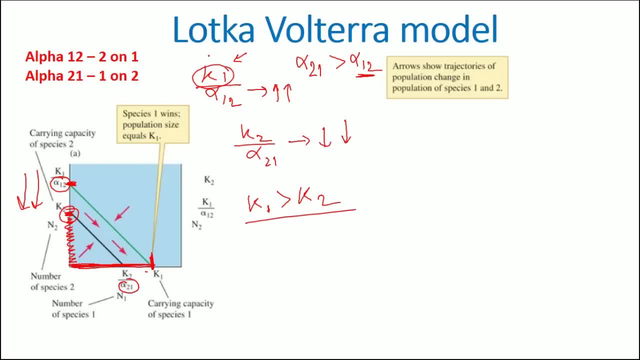 environment is favoring species number one. So in this case, species one wins. and that's the beauty of this graph, Because in all this graph, the one will win for which the isocline value or the graph will be on top. In this case we see the value for species. one graph is on top of species. 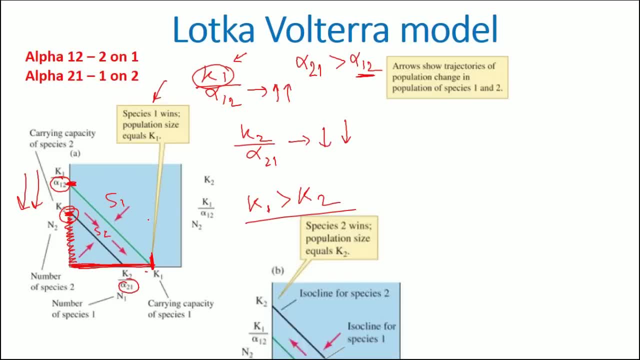 two graph. That's why we see species one is winning In the second situation. here you see that the graph for species two is on top than species one. Now again, if we calculate it here, value for K12 by alpha 21 and K1 is equal to K2.. So K2 is equal to K1 by alpha. 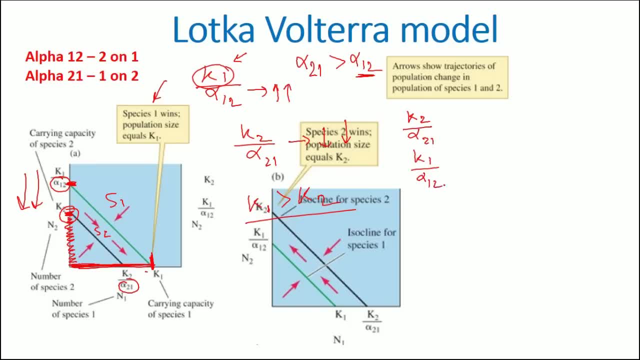 21. So K2 is equal to K1 by alpha 21. So K2 is equal to K2 by alpha 21. So K2 is equal to K1 by alpha 21.. Now what we are seeing here, alpha 12 is more than alpha 21.. So in 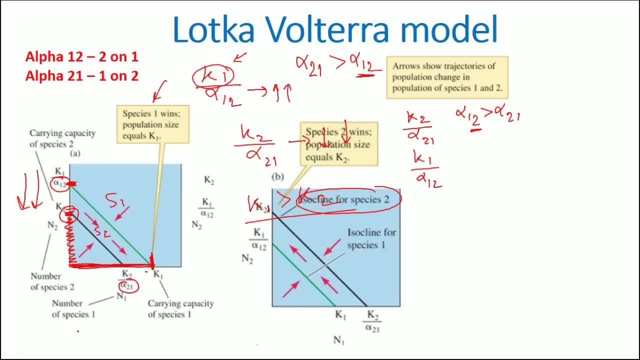 this case, the value for K2 is going to be more than compared to the value for K1. If you look at here, the value for K2, that is, the carrying capacity of species two, is far more Species one, which is only this. So as K2 is much more than K1, we know K2 is going. 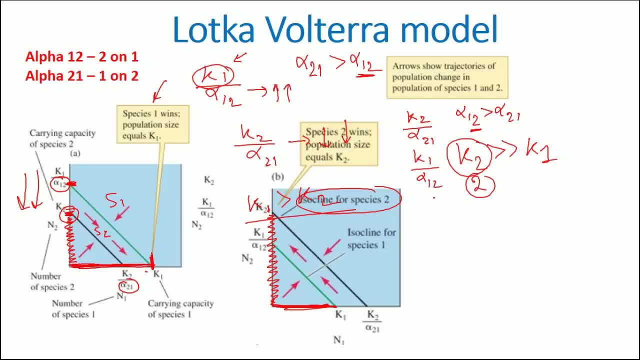 to win, That is, the species number two is going to win. Right, And again based on that same idea, that in this case we see the isocline, of species two on top. So that is going to win. So, as we know this, graphs can be placed in a way. in every single case, the one will. 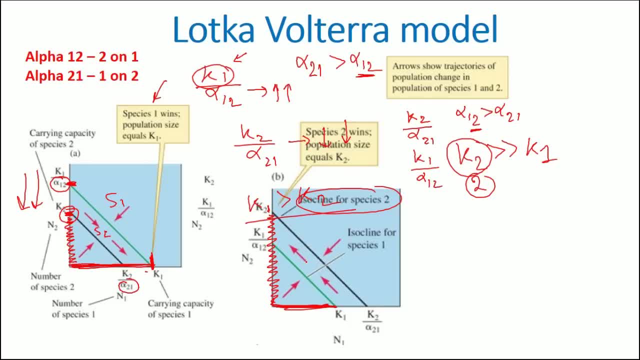 come on top, The isocline, for which species will get on top. So that is going to win. So, as we know, this graphs can be placed in a way: in every single case, the one who will come on top is going to be the one who will win. 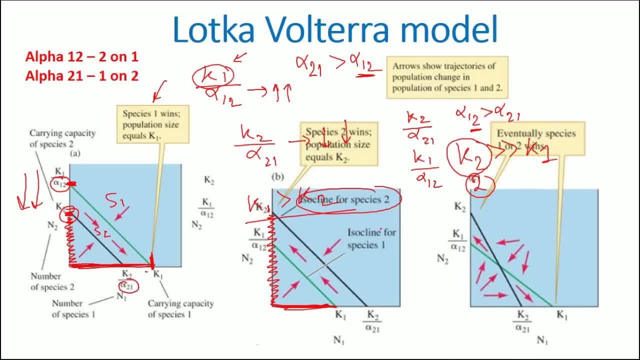 There is a third situation where, due to the alteration of the value for alpha 12 or alpha 21,, the idea behind the values of K1 and K2 is not well understood. Well, both this isoclines intersect each other in a point. Now they can move in either of this direction. In this, 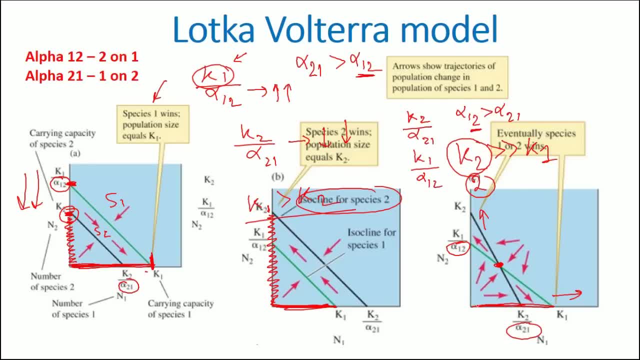 case, you will calculate the K1 and K2. So K2 is going to be the one who will win. Now there is a third situation where, due to the alteration of the value for alpha 12 or alpha 21,, the idea behind the values of K1 and K2.- So this time K1- is not well understood. 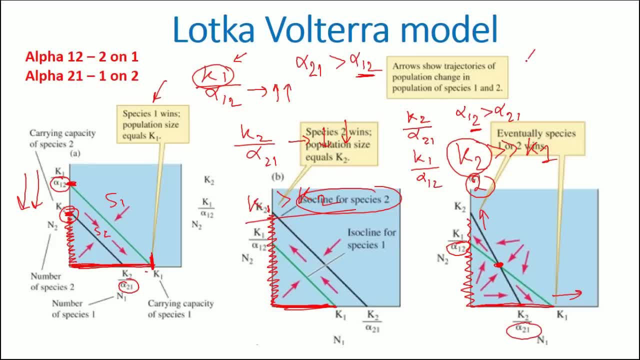 In this case, it will come on top. So the idea behind the values of K1 and K2 is not well understood. Now, either right way or left way, Let say where the stayed, as isocline has a sign, not showing a fingers. Next, there is a third situation where, due to the alteration, of the value for alpha 12 or alpha 21,. the idea behind the values of K2 is not well understood. There is a third situation where, due to the alteration of the value for alpha 22,, the idea behind the values of K1 and K2 is not well understood. Then we cannot do prediction or 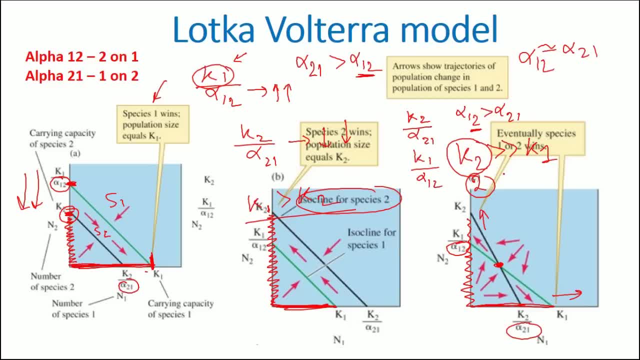 any indication. Two: you know the general concepts I had mentioned earlier features. this undred opposite as positions is called proof right. OK, You will see that you have to valid Mortal Species 1 or Species 2 Can Win Because Both Have the Capability of Win. That Is How We 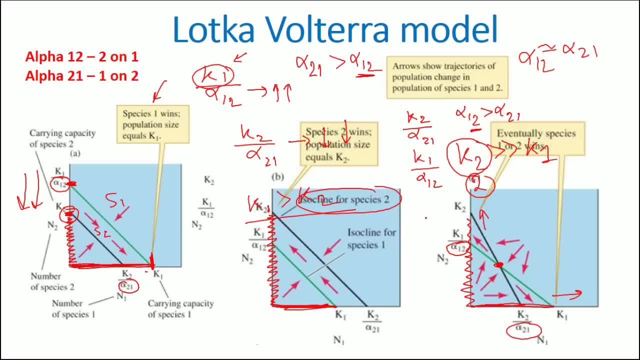 Predict You Can, Volterra Model and With the Help of What Can, What There Are More. We Can Predict the Predator, Pre Relationship. We Can Say Whether Species 1 Is Going to Be Predator or Species 2. Okay, So Now, As We Know About the Lotka Volterra Model and As I Making This, 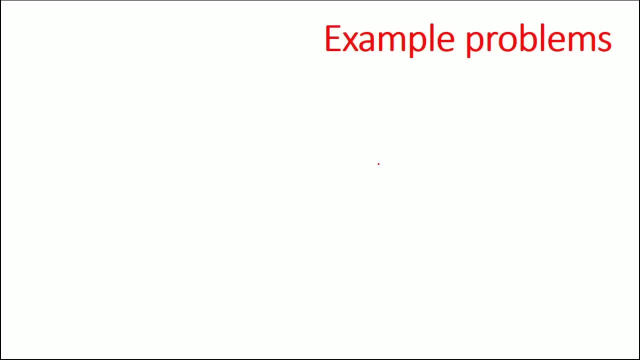 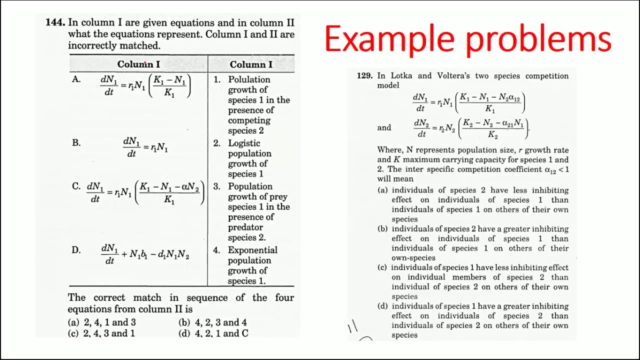 Video. Keeping in Mind That This Question Asked from This Region in CSI NET Exam, I Put Two Separate Questions So That You Get to Know What Kind of Question They Generally Asked from Here. See the First Question. It Says You Have to Match Column 1 with Column 2. Now Look. 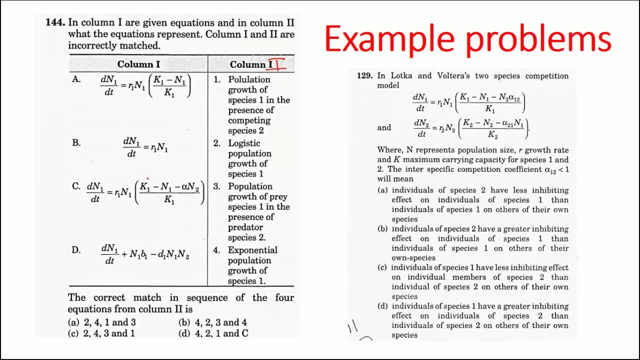 at Here in the Column 1, There Nothing but Different Equations Provided, and If You Look at Here in This Video, We All Already Talked About Three of Those Equations. Already We Talked About This Equation, This and This in This Particular Video Itself. 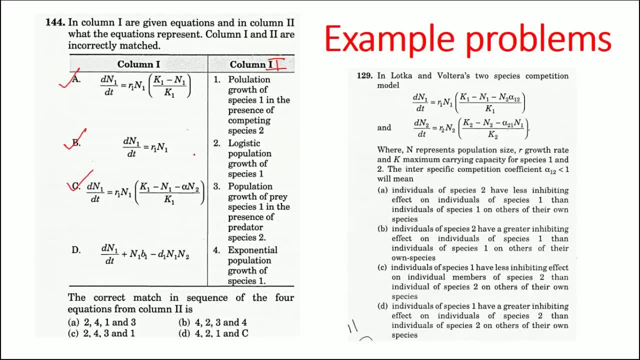 So, As You Know Three Out of Four Equations from This Video, I Think You Can Solve This Question Quite Easily. It Says: DN 1 by DT equals R 1 and 1. This, We Know, Is a Graph for Exponential Growth. So It Will Match with 4. Then This One, While We Involved Carrying Capacity but No Carrying. 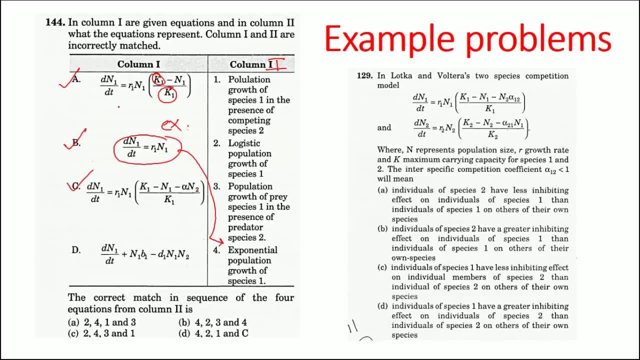 Capacity. It Will Match with 3.. So This Is It. It Is No Capacity. and That Will Be the Second Question. Now Let Us Look at This Question Again. So Let Us See This Question Again, Question 3.. What Is the Compatibility? 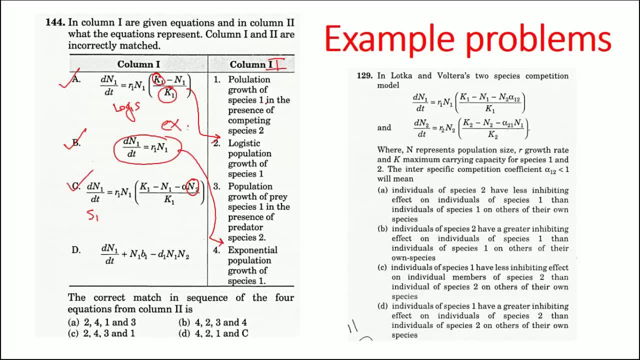 Species 1 in the presence of Predator Species to Population. Growth of Species 1 in presence of competing Species to Predator Species or competing Species to. with the help of this particular formula, We cannot predict whether Species 1 or Species 2 is going to be competitive. 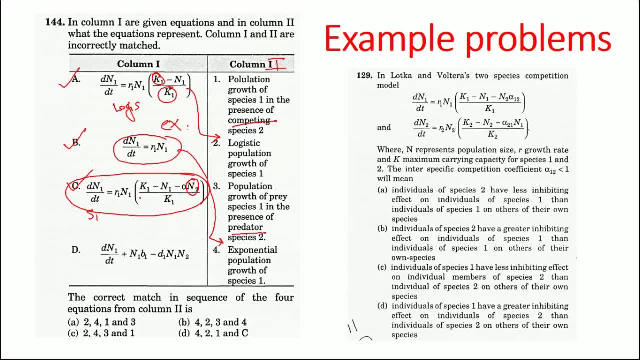 Predator of Prey. We simply know that Species 1 and Species 2 are in competition. It can be Predator, Prey or may not. We don't know exactly who is Predator and who is Prey. So it's the best way to select competing Species. So Option 1 from there. So while we tag with, 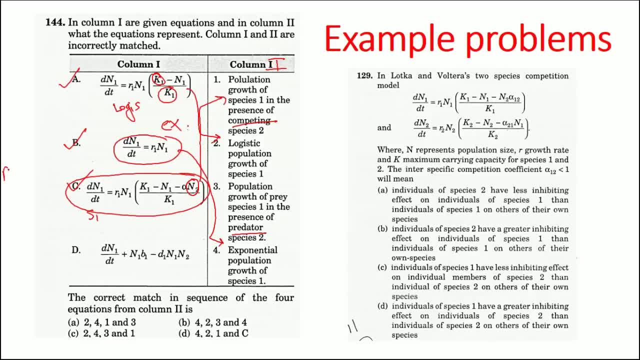 remember we're tagging here with A with 2, B with 4 and C with 1.. So, based on A, B, C, D, what we can put: 2, 4, 1 and 3.. So 2, 4, 1 and 3 is the Option A. 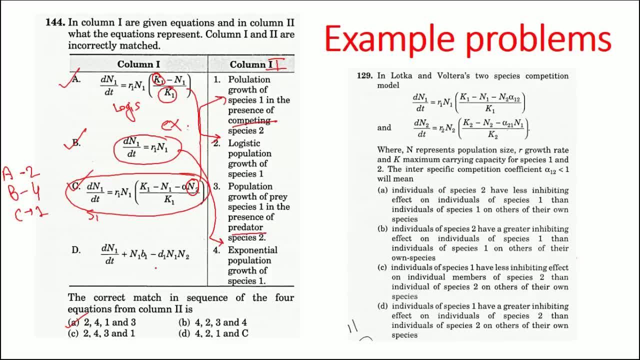 That is going to be the correct one, Because D will be tagged with 3.. Because it's what remains here. That's how we can answer. To predict whether the competitors are Predator or Prey, we need to look at the graph, Otherwise we cannot tell it. For the second problem: 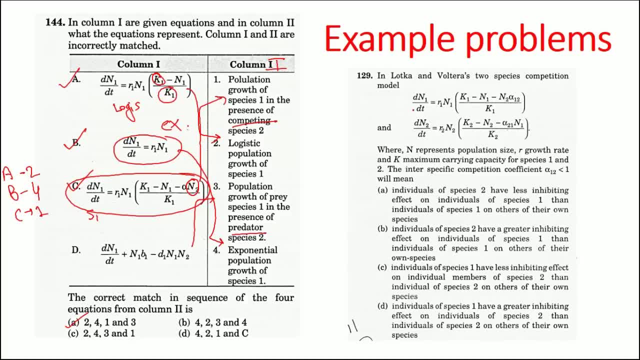 here we will see two Species in competition and the growth for both. the Species are given And it says: where N represents population size, One growth rate and K maximum carrying capacity of Species 1 and 2.. The inter specific competition coefficient, Alpha 12, is less than 1.. The value of Alpha 12 less than 1 signifies the impact. 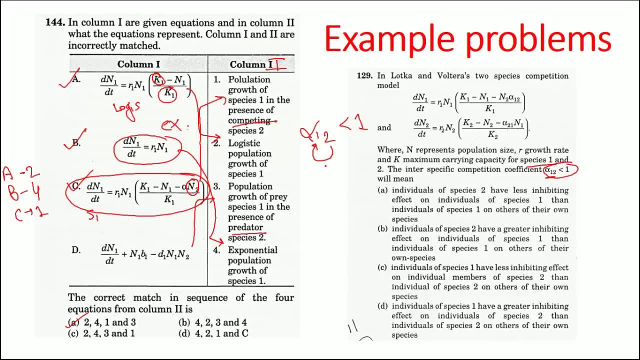 of Species 2 on 1 is comparatively less compared to the impact of Species 1 and 2.. So in this case it is telling you Alpha 12 is greater than Alpha 21.. So either they tell you like Alpha 21.. 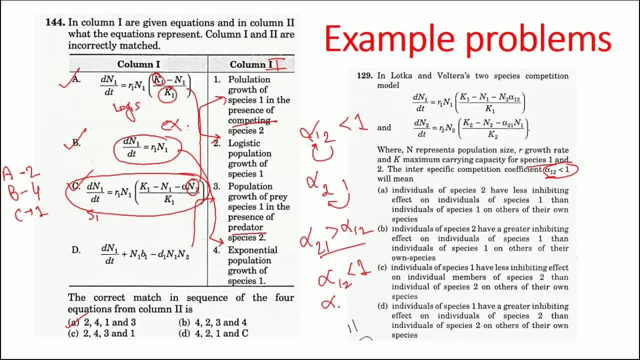 Or they say Alpha 12 is less than 1, or Alpha 21 is greater than 1.. They all mean the same thing. So here, which among the following is the correct option: individuals of Species to have less inhibiting effect of individual of Species 1 than individual of Species 1. 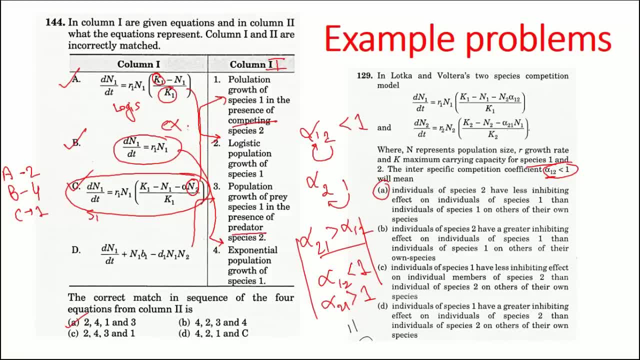 and other of their own Species. that sounds quite of correct, because individual of Species 2 impact on Species 1 will be less compared to 1 and 2.. Species 2 have greater inhibiting effect on individual of Species 1, that's not going.